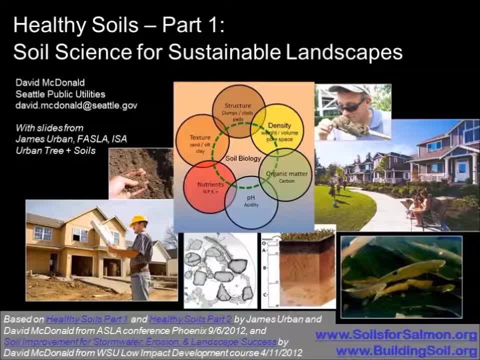 Healthy soil is the foundation of a sustainable landscape, A landscape that looks good year-round and is healthy for our environment. Hello, I'm David McDonald. I'm an environmental scientist at Seattle Public Utilities And this is the first part of a two-part class looking at healthy soils for landscape professionals. 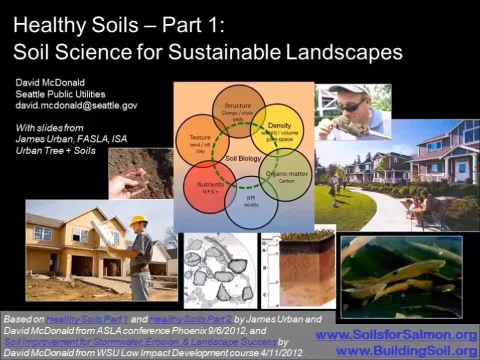 In this first part we're going to look at basic soil science concepts that are useful to landscape professionals, And the second part, we'll put those concepts to work to protect and restore and maintain healthy soils throughout all our projects. You'll note that there are internet links on a lot of these slides. 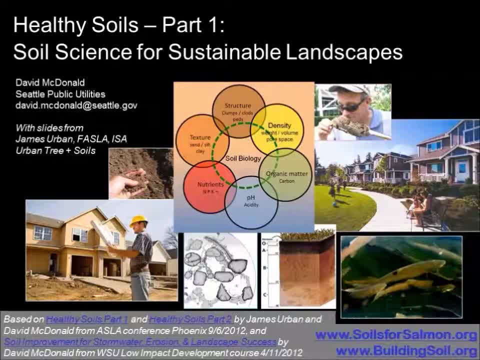 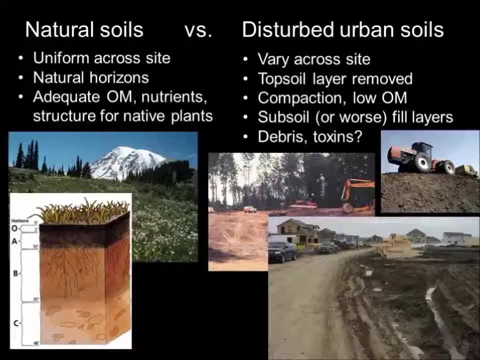 And those links are all available in the resource handout, which is on the same website with these slideshows. The first thing to know when talking about soil science is: most of our soil science is developed around natural soil conditions, Soils that have undisturbed horizons and natural deposition layers. 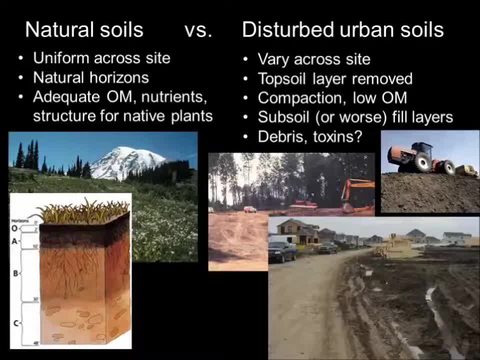 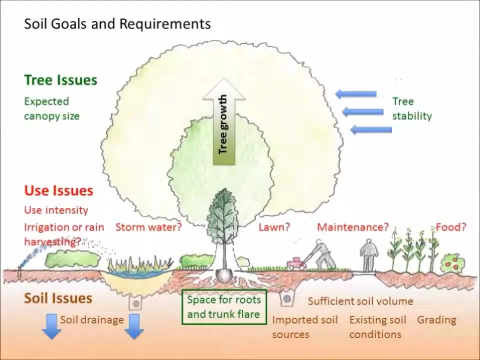 And, in general, soils that are adequate for the plants that are growing on their site, Whereas as landscape professionals, of course, we mostly work in disturbed soil conditions, which can have a lot of changes over time. The other thing to think about as you think about this soil science and how to apply it in your sites. 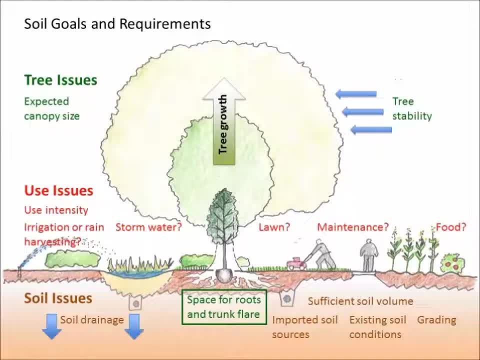 is how that site is going to be used and what the requirements are for the soil. on that site You might be growing large trees, You might be growing turf or lawns, or a conventional landscape or a restoration landscape, a stormwater system, a food garden- a variety of uses. 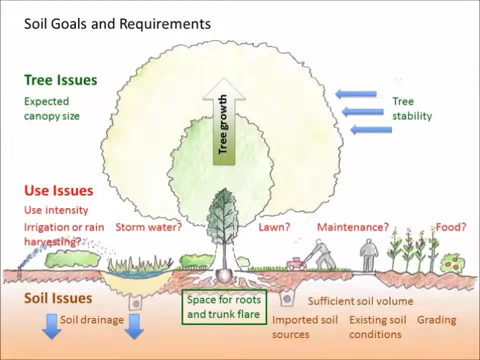 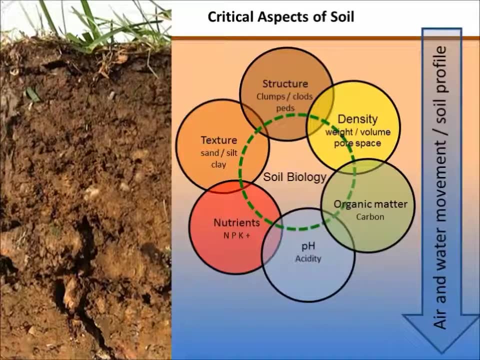 And obviously your soil landscape And obviously your soil needs are going to vary for each of those uses. So these are some of the aspects of soil that we're going to look at in part one of the class here: Soil texture, structure and density. 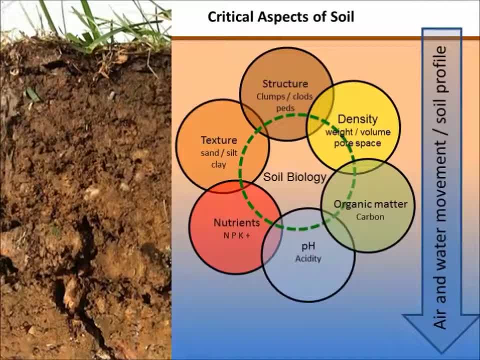 Nutrients, pH, acidity or alkalinity, Organic matter, both living and dead organic matter, And then, of course, the soil biology that ties all that together and, as we'll discover, actually creates most of the functions that we care about. 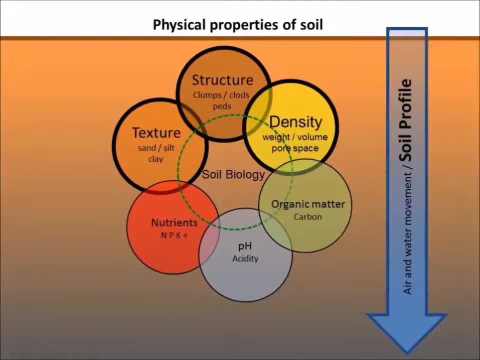 In the soil. So for the first part, we're going to talk about physical properties of soil, particularly what's known as texture, structure and density, And scientists use those terms in a particular way which is not exactly the same as we use them in plain English. 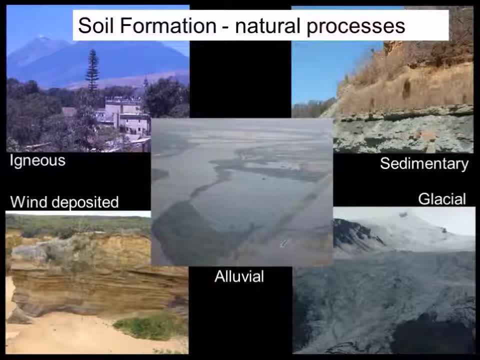 So we'll try to explain that as we go along. And before we get into those soil physical properties, we'll look for a moment at the way that our soils are formed. There are obviously a variety of sources or depositions or manners in which soil layers can be created. 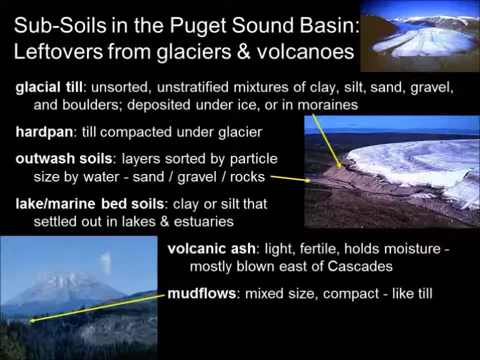 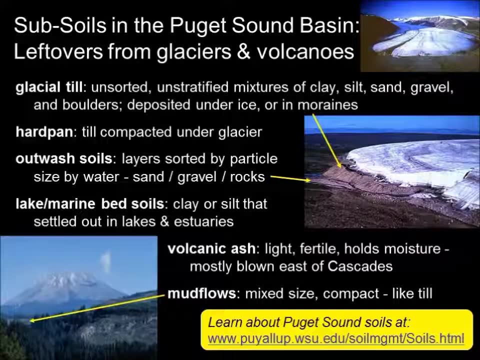 And here in Washington most of our soils are leftovers either from volcanic activity or from the glaciers that came one after another over the last hundred thousand years or so, And you can learn a lot more about Washington soils at the Washington State University Soil Management website. 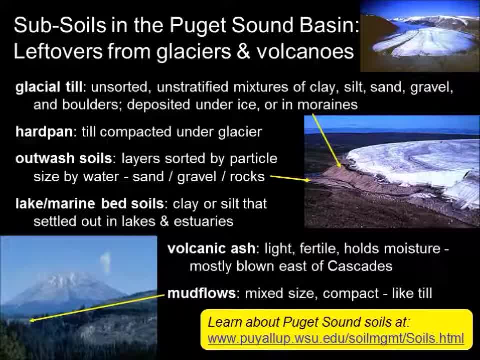 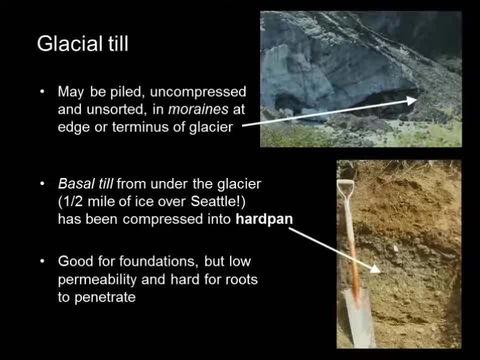 which the link is on the screen, Or you can just Google WSU soil management and that will get you there. We have a variety of soils left by glaciers. Probably everybody has heard of glacial till. Glacial till is just the unsorted material, various sized, you know. 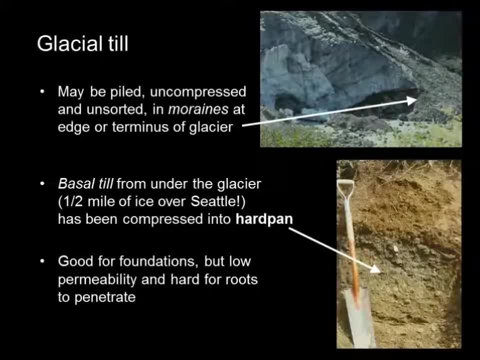 from silt to sand, gravel to stones that are pushed up and ground up by glaciers. They may be left in a loose state as a moraine at the edge of a glacier. Or more commonly, here in the Puget Sound Basin, we see them as basal till, that is, glacial till that was compressed under half a mile or more of ice. 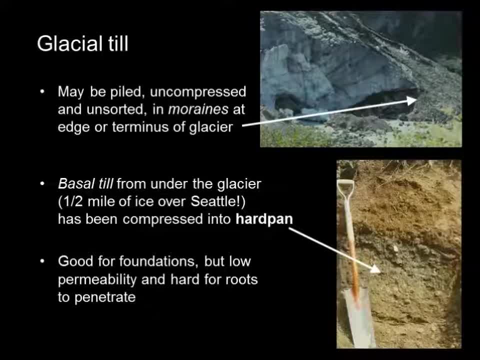 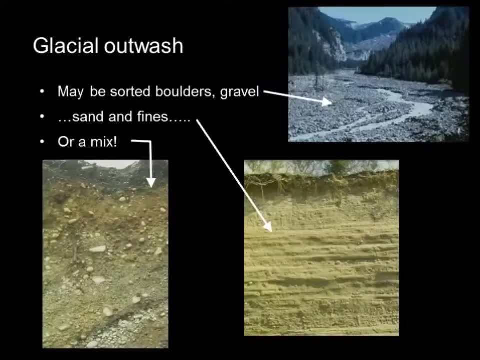 so that it became kind of like concrete. So, as you can imagine, this concrete-like material is great for foundations, but it has low permeability and it's hard for roots to penetrate. Glacial outwash soils are created as glaciers retreat, and the melting water carries stones, gravel, sand, silt and clay on downstream. 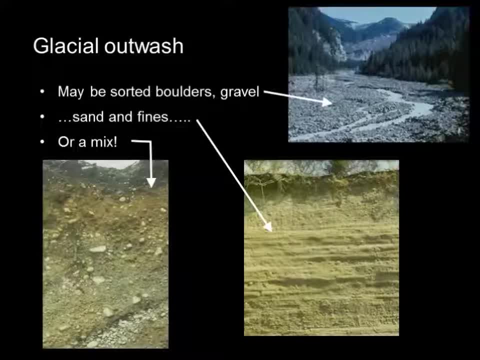 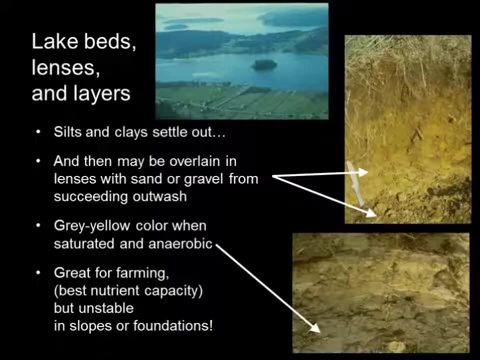 obviously dropping out the biggest particles first and then smaller particles as the water slows down And as that water slows down even more into still bodies of water like lake beds. the very finest particles will settle out- fine silts and clays, and those are high in nutrient holding capacity. 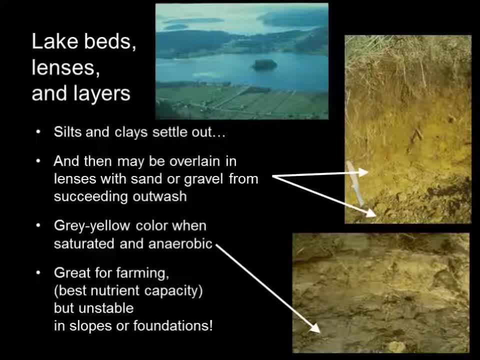 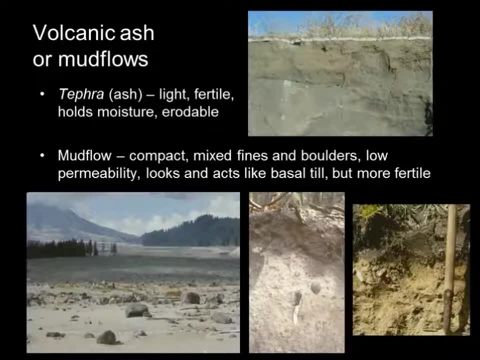 but difficult for air and water to penetrate. Here in western Washington we have a lot of mud flows that came down from our nearby volcanoes when they blew up, when they were topped with glaciers, and that water melted and turned to mud and carried all that stuff down the slope. 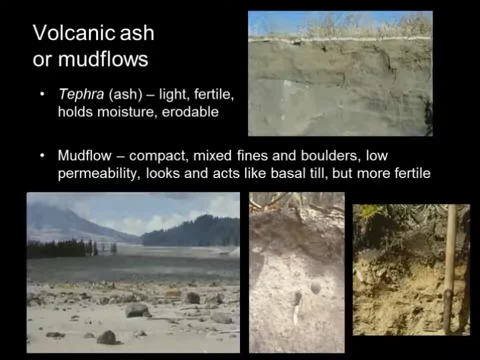 Over in eastern Washington, because that's the direction the wind was blowing when they blew up. we have a lot of volcanic ash soils. These soils are high in nutrients, but they can also be quite compact and difficult for air and water to penetrate. 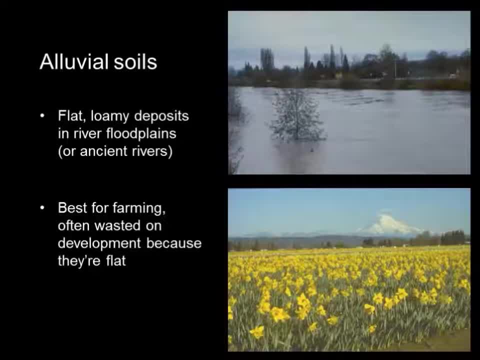 And then, as the rivers flowed down and flooded out over flat areas, they deposited intermediate textures of particle sizes that we call silt. So this is sort of intermediate between sand and clay, clay being the finest The silt that settles out in our river plains is great for holding nutrients. 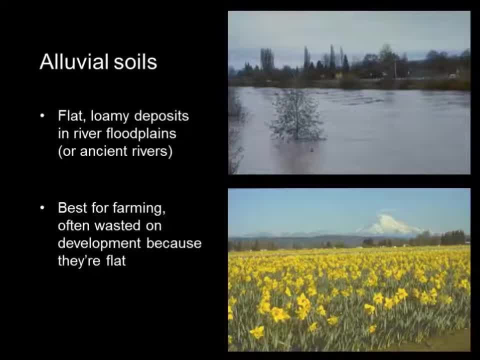 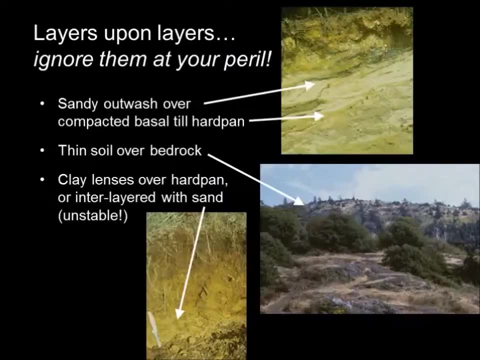 and good for growing on. Unfortunately, we also oftentimes tend to like to use those flat grounds for putting warehouses or housing developments on. We get many layers in our soils in Washington caused by volcanic ash flows, by different glacial periods, by flooding and outwash activities. 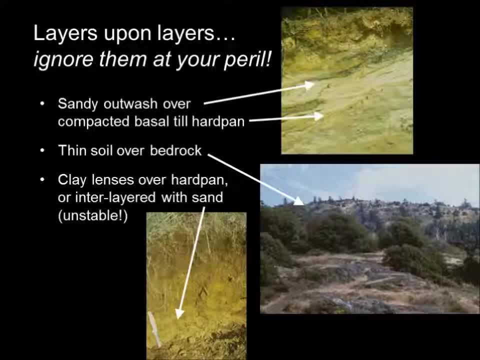 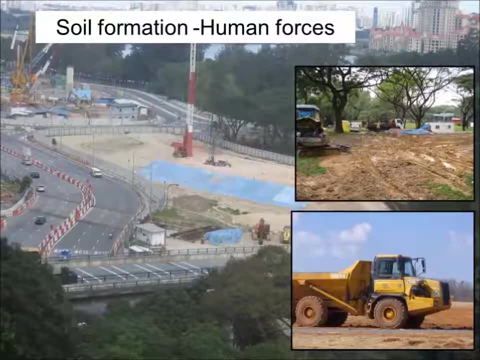 And so we may often have layers that appear somewhat confused, one on top of another. Very important to pay attention to those layers. And then we have the forces, our human forces, that actually create a lot of the soils that landscape professionals deal with. 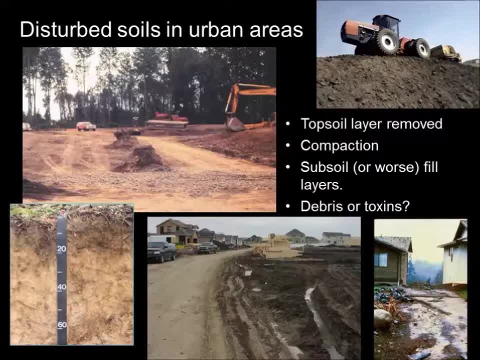 where we scrape off and compact, And for instance in our urban areas, we've oftentimes removed layers of soil. In this top left picture you can see where they've removed about three feet of soil on that site and compacted the rest. 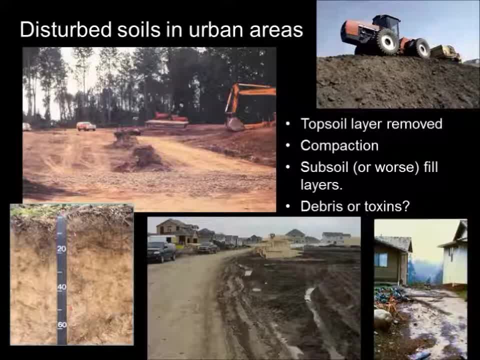 So they've removed most of the topsoil or all of the topsoil, and compacted the subsoil, which makes a very difficult growing medium. We also oftentimes have toxins or other sorts of spills and things that have contaminated soils. 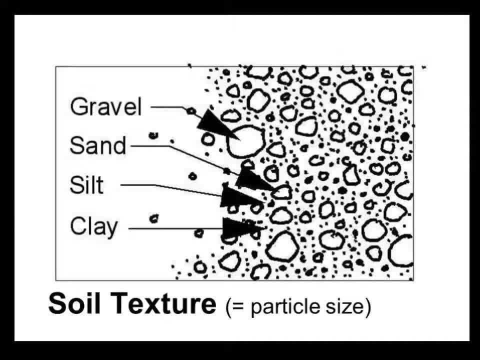 So now, digging into our soil science, we're going to talk about the first term and classification way of looking at soils that soil scientists use, and that is soil texture. And what the scientists mean by that is the particle size, And specifically when they talk about soil texture. 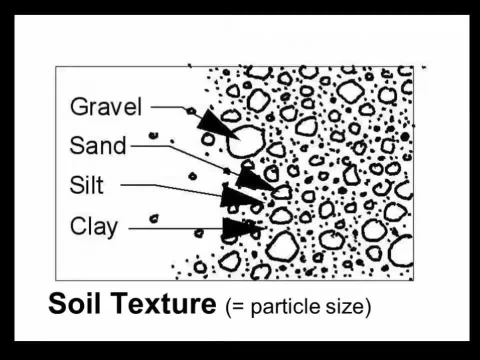 they're referring to these three sizes: sand, silt and clay, sand being the largest and clay being the finest microscopic that we find in soils, But of course there are larger particles in soils too: gravel, small stones, large stones, big boulders. 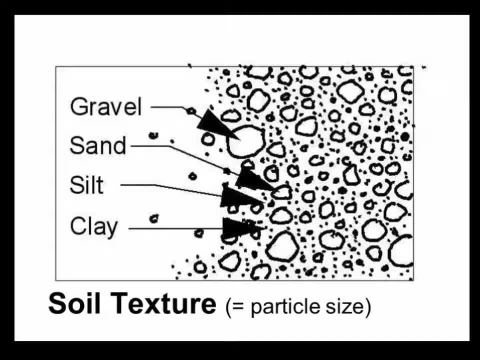 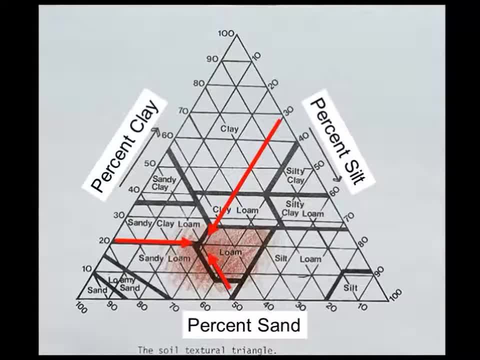 So all those things are part of soil texture, Although when we do a soil texture analysis we really just count the sand, silt and clay Soil. scientists use this soil texture triangle to represent that, with the percent clay being on the left. 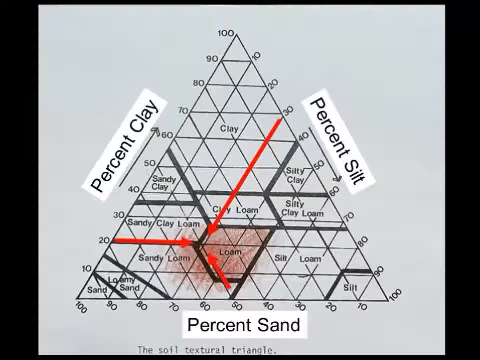 percent silt on the right and percent sand across the bottom. And there's sort of a sweet spot in the lower center there that scientists call loam, where you have an ideal amount of sand, silt and clay for growing. But whatever your soil is sand, silt or clay. 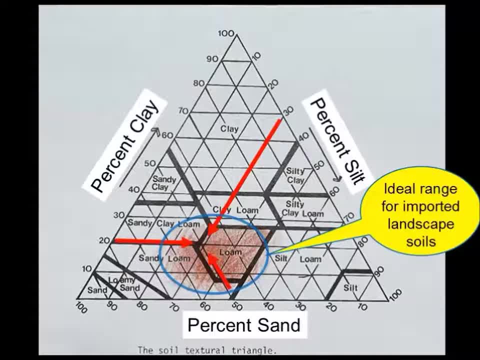 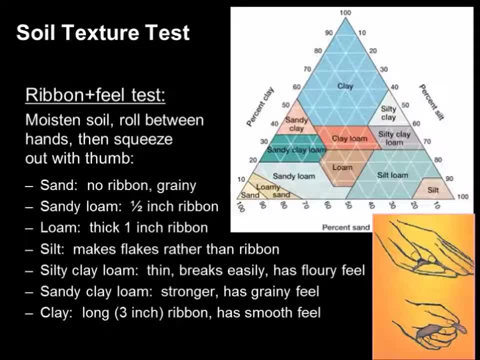 perhaps without a lot of admixture of the other size fractions. you can improve that soil with organic matter and we'll be talking about that more. To do a soil texture test in the field, you can just take some soil, moisten it. 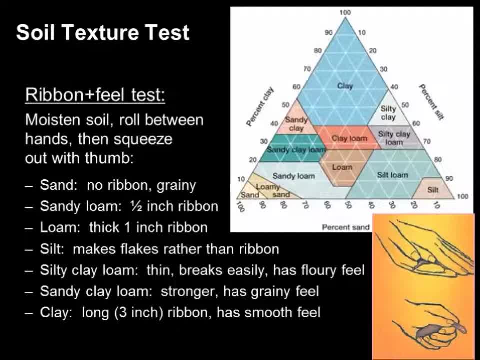 rub it between your hands and then roll out a ribbon. to see how long a ribbon it will make And that will help you determine how much sand, silt and clay your soil has in it. To see a great video, Dr Craig Cogger showing you exactly how to do the soil texture test. 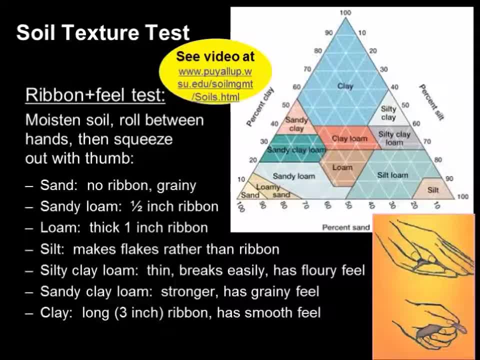 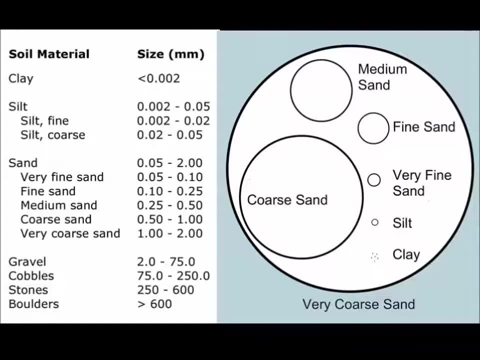 go to wsusoilmanagementcom, the WSU Soil Management website. Again, if you just Google WSU Soil Management, you'll get there or follow this link, And it's important to understand that there are really huge size differences between these different particle sizes. 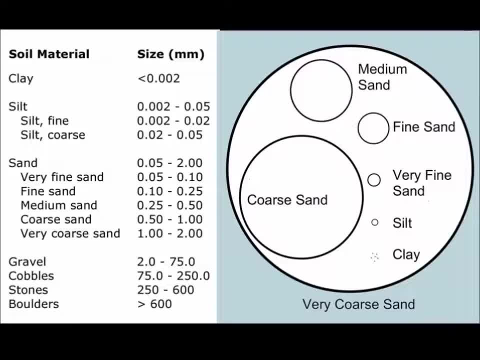 You can see represented on the screen here about what the coarse sand looks like and then the tiny dots of clay particles with the smaller silt in between. This silt is almost microscopic and clay particles are microscopic. They're little flat, microscopic plates actually. 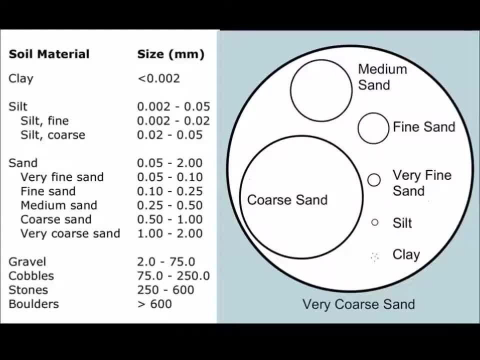 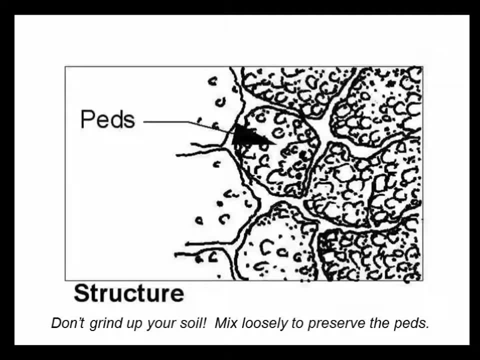 So this is important when you think about soils, because those particle sizes actually vary. And then the other thing that we actually see when we look at soil is not so much those individual particles but what soil scientists call PEDs, which are the clumps of soil. 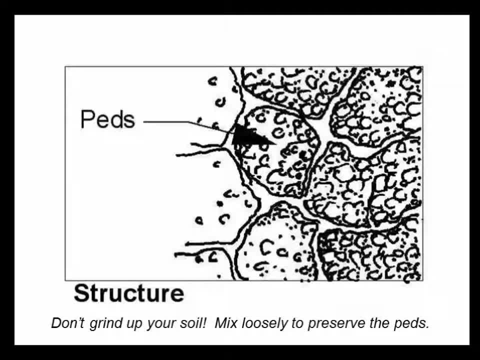 If you dig up a shovel full that breaks in your hand or on the shovel you may have PEDs that range from a quarter inch in diameter to several inches in diameter, And these are sort of the largest level of soil structure in the soil. 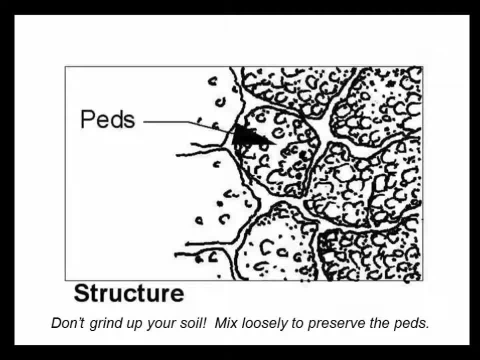 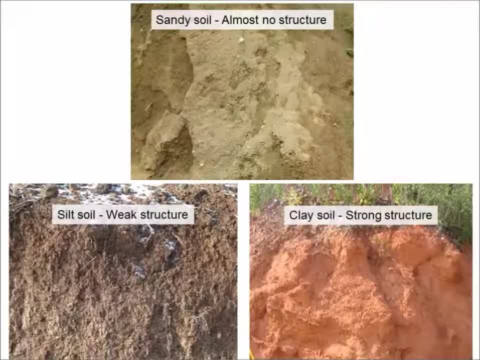 and they're something we like to preserve, which is why we say: don't grind up your soil, Mix it loosely to preserve the PED. Now, soil structure in these mineral components depends on which of those size particles it is. Obviously, sand falls apart easily. 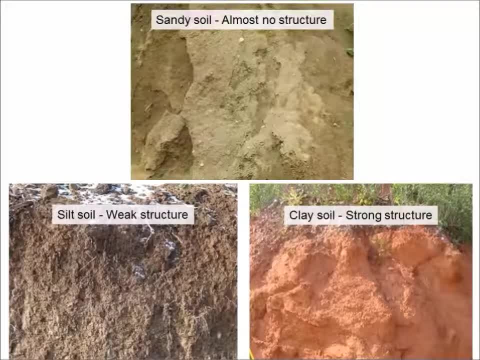 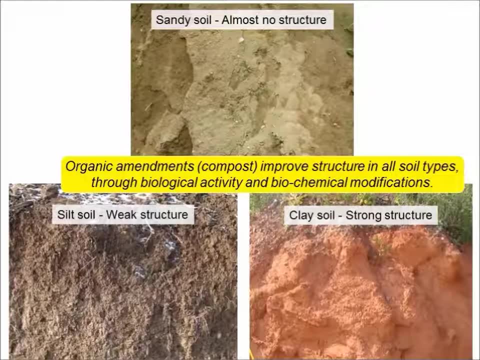 Silt sticks together somewhat and clay sticks together a lot. However, we can improve the structure of any of these soils just by adding organic amendments, specifically compost, and we're going to talk more about that. It's really the biological activity over time. 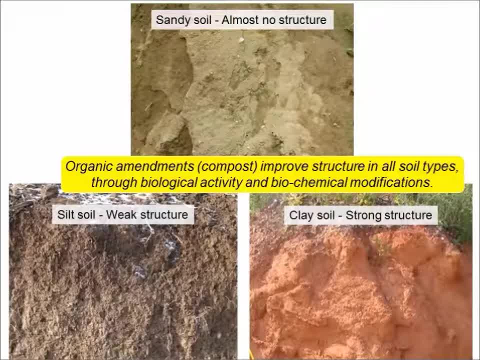 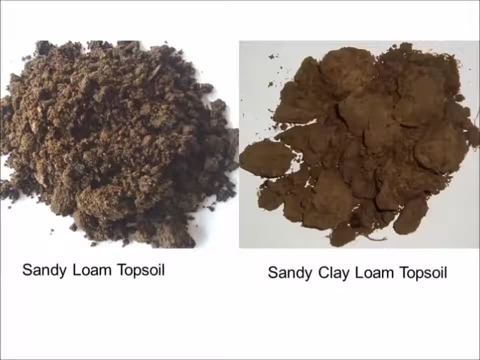 in the organic matter that creates soil structure that we care about. Here's an example of a sandy loam topsoil. as opposed to a sandy clay loam topsoil, Obviously you can see larger PEDs, more cohesion in that soil that has some clay in it. 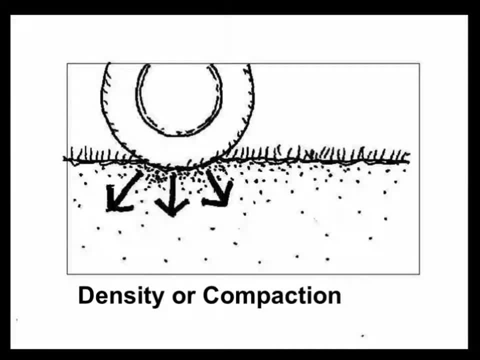 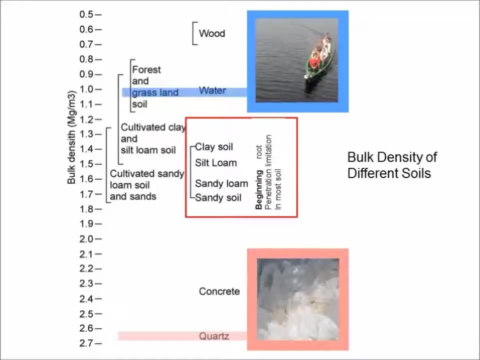 The second concept, after texture, that soil scientists talk about is density or compaction, And what they mean by density is how much it weighs per unit volume, and that's really more than anything has to do with how much pore space it has in it. 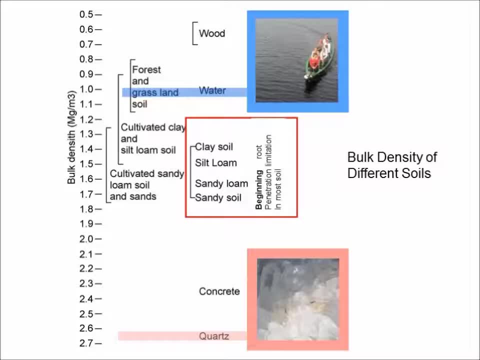 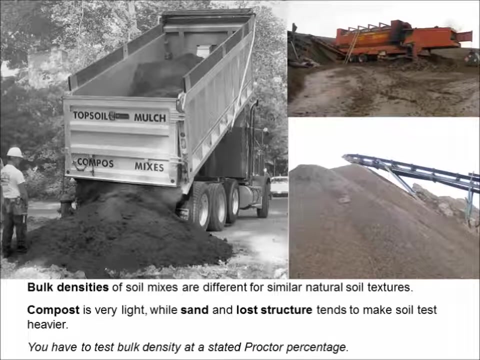 Here's a chart that shows relative densities of some different products, from stone at the bottom to wood and water up the top and in between some of our soils, with pure sand soil being the densest and a clay soil being lighter because it actually has more pore space. 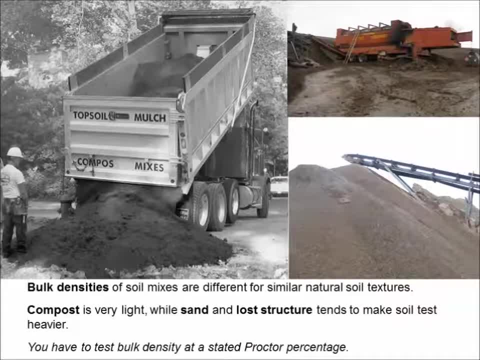 The bulk densities of different mixes that you might buy vary a lot from natural soil textures. It's important to recognize when you're mixing soil that compost or the organic matter you might add is very light, while sand and compacted soils obviously are much denser and heavier. 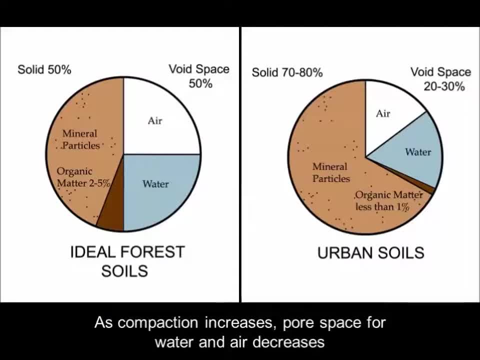 As that soil compaction increases, we lose the pore spaces that allow air and water into the soil And you can see on the left sort of an ideal soil condition where about half the soil is pore spaces that are full of air and water, whereas in a compacted urban soil condition. 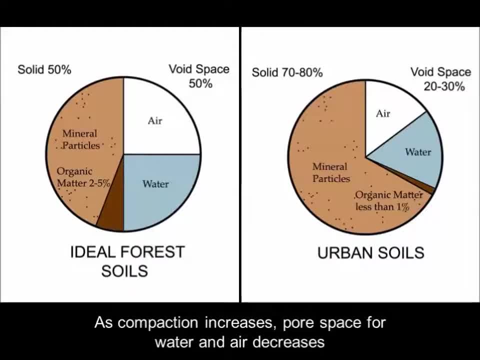 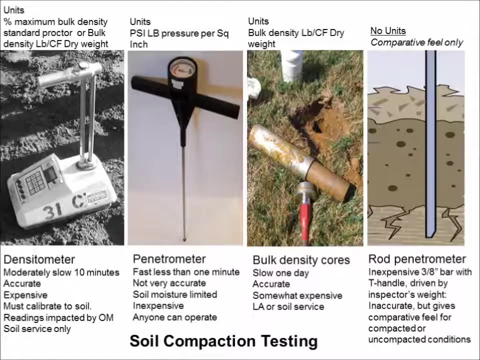 your void space or pore space may be as low as 10 to 15 percent, So it allows much less air and water into the soil. It's also harder for tree roots to grow in it, harder for the soil biology. There are a variety of tools shown on the screen here. 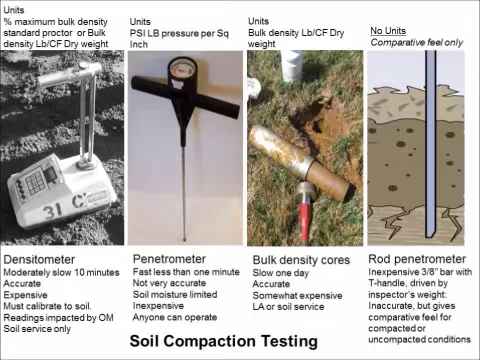 that you can test with From most expensive and most difficult to use, the nuclear densitometer on the left. the gauge penetrometer, second from left, is actually a tool that you might want to own and use in the field. You can get a pretty accurate reading. 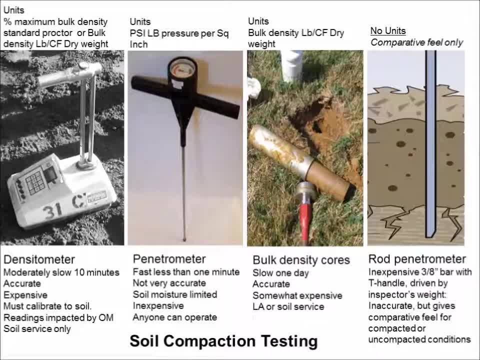 if you use it repeatedly in the same soil types. but individual readings tend not to be very accurate. You can also take a soil core and send it to a soil lab. You need to follow a very strict protocol. That test is fairly accurate. 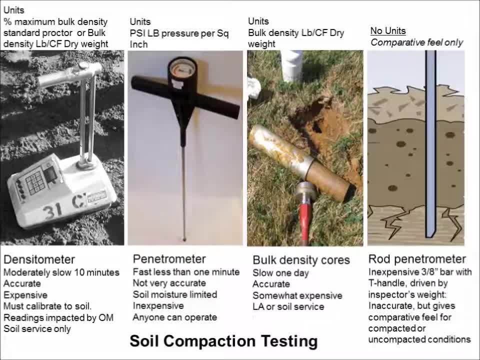 but the tests are slow and expensive And you can also just use a shovel or a rod that you push into the soil And for you as landscape professionals, this is a good tool to use on all your sites to start to get the feel of what the relative density is. 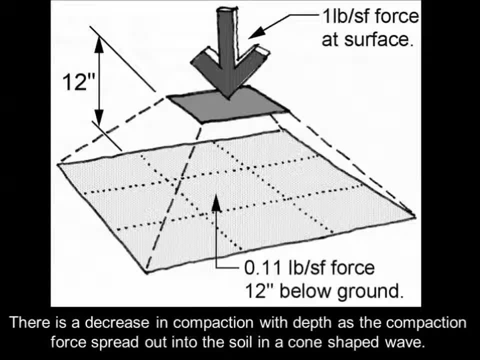 or compaction of the various soils that you're working on. It's also important to note that, because we load up the soil at the surface, whether it's a glacier pressing on it or, more commonly, in our urban environment, feet or trucks or whatever- 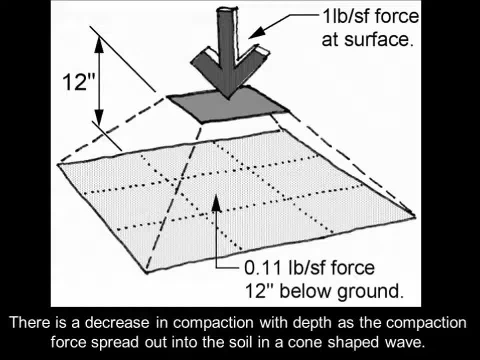 we compact the soil closest to the surface the most, because that weight or pressure spreads out as we go down. So you're going to get your most compacted soil nearest the surface, which is nice for us because that's where it's easiest for us. 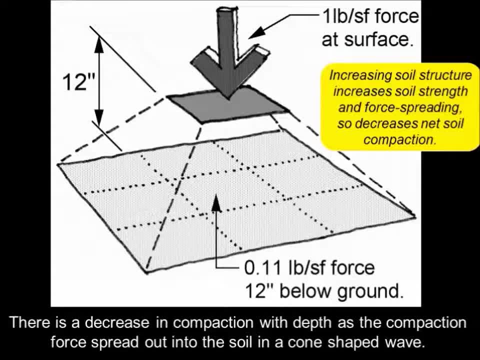 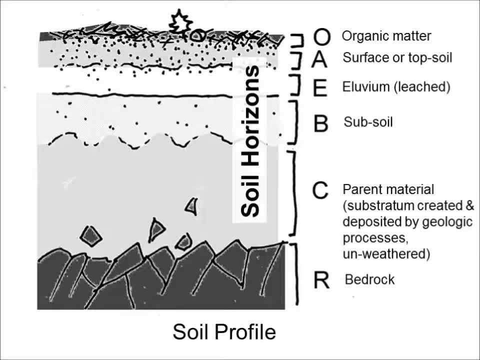 to fix over-compacted soil. These are the natural soil horizons that soil scientists talk about, with organic matter or duff at the top, The top soil horizon: A horizon, sometimes a leached layer underneath that, but then certainly a subsoil. 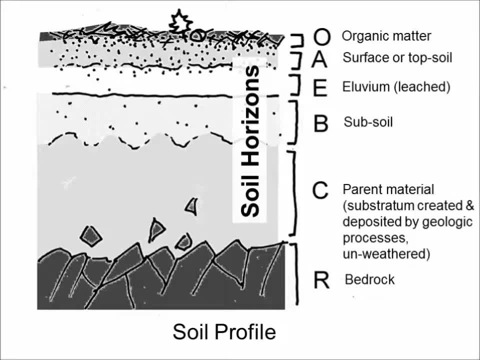 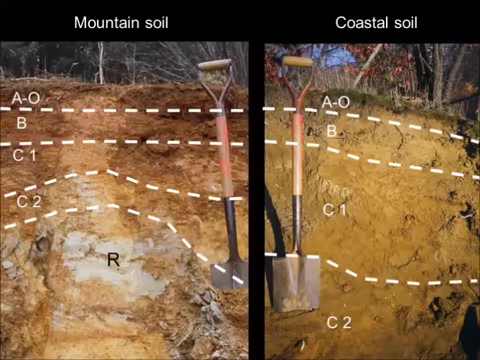 which is somewhat biologically modified, And then underneath that, the parent material, basically, whatever the glacier shoved around And underneath that you might find bedrock, if you're in an area where there is bedrock, And these layers can vary widely depending on where you are- 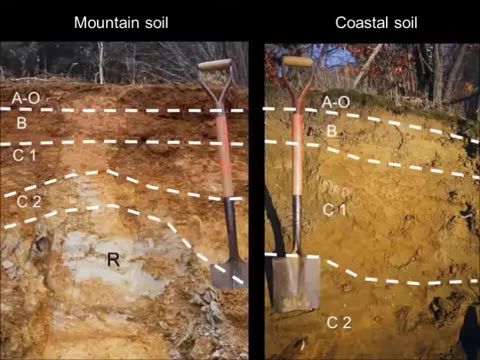 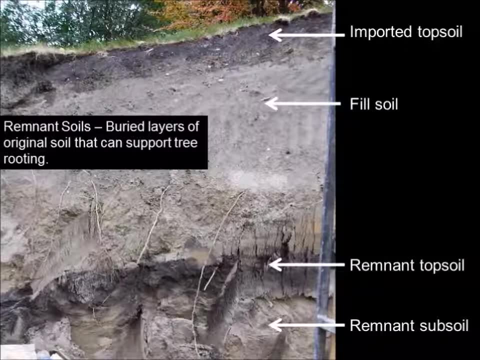 So digging a hole and taking a look is always a good idea. In our developed environment we actually can oftentimes see soils that are broken up into layers that don't immediately make sense. Here we have down at the bottom that dark layer which is a remnant topsoil. 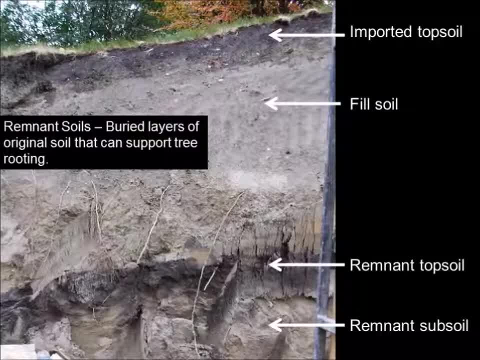 and then above it is a big layer of sandy soil and then some pretty clay soil that was dumped on top of it, and then some imported topsoil dumped on top of that. What we see in this case is the tree roots have tried to find their way down. 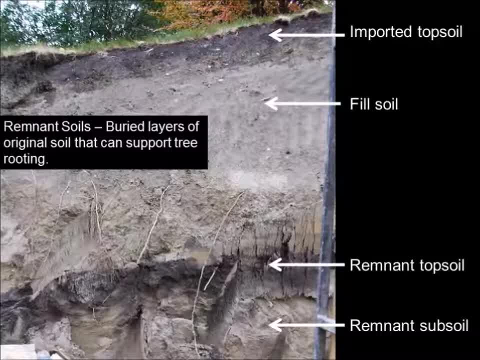 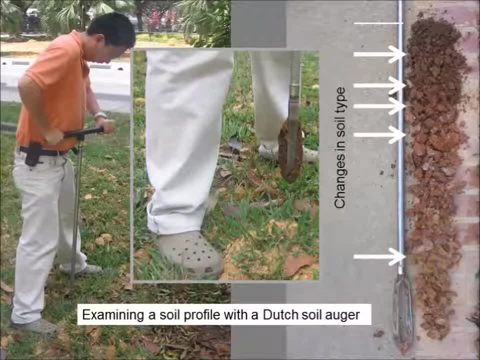 to that high-quality remnant topsoil, So you'll oftentimes see them seeking out wherever the good soil layers are. This is a tool that is really great to have if you're a working landscape professional or landscape architect designer, to really dig in and take a deeper look at your site. 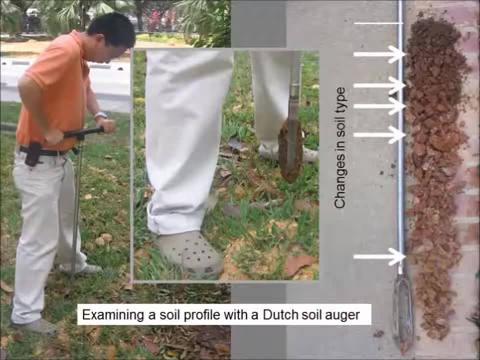 This Dutch soil auger can be extended for several feet and you can drive it down into the soil by twisting and actually pull up a soil column in several layers going three to six feet deep and actually see what's going on in that site. So it's a very handy tool. 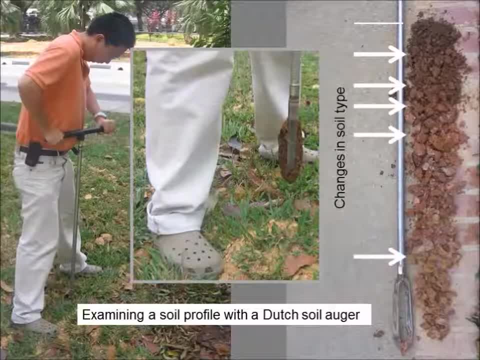 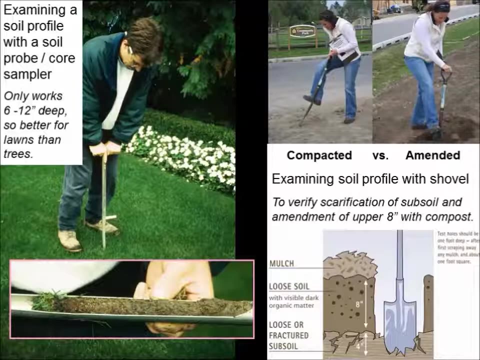 The simpler soil core sampler that you can buy at most landscape supply stores that goes a foot or so deep is really an indispensable tool to have in your toolbox. Here we show that simple soil core sampler on the left or on the right, just using a sharpshooter spade. 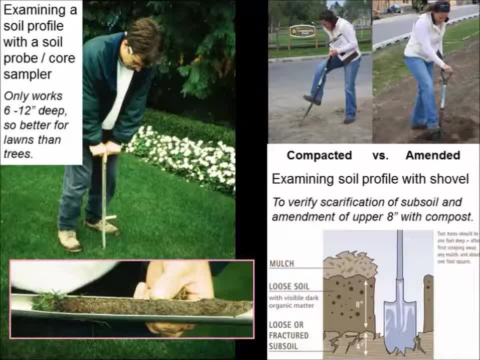 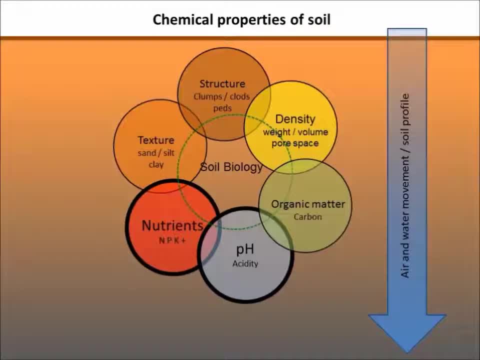 to dig a pit and compare soil conditions. So that was our discussion of soil physical properties. Now we're going to talk about chemical properties, specifically nutrients, including cation exchange capacity and pH or acidity, alkalinity. You'll see that these things are related. 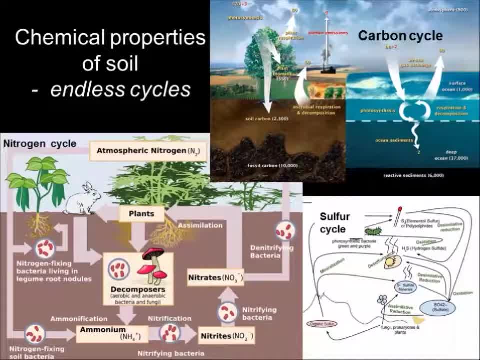 The important thing to understand about the chemical properties of soil is that they're not fixed. They change both over the long term and relatively quickly. For instance, everybody's familiar with a compost pile or soil that has become anaerobic and stinky because air has been excluded. 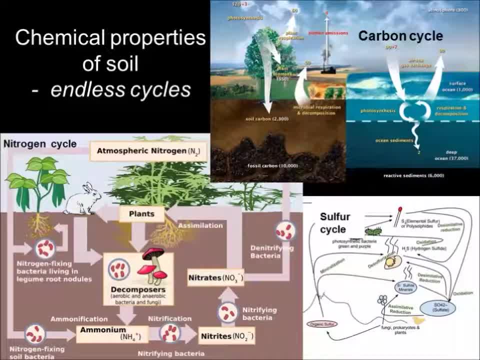 by being too compacted or covered with plastic. And when you loosen that soil up and let air into it, that actually changes the pH of the soil because you get aerobic bacteria going in there so it becomes less acidic And that changes the chemical interactions. 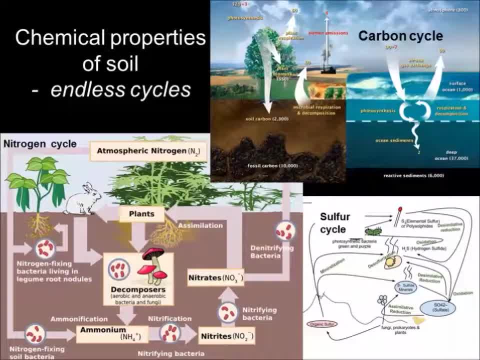 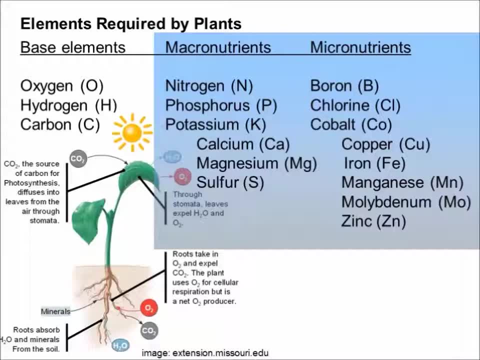 in the soil. And then all that soil biology is really what's mediating these soil chemical cycles over time? Plants need a variety of nutrients, just like us, And just like us, the majority of their body is made up out of chemicals from the atmosphere. 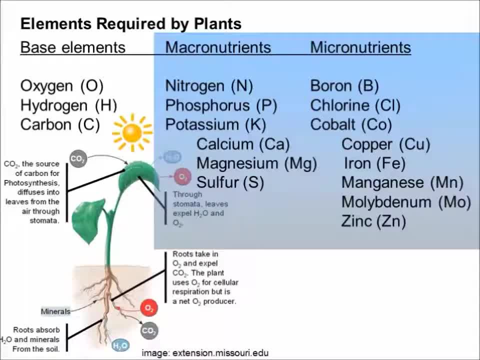 Oxygen, hydrogen and carbon. So we, of course our bodies are percent. water Plants are about the same: Their oxygen and hydrogen and carbon, carbohydrates, amino acids. They also need a bunch of other nutrients, The ones they need a lot of. 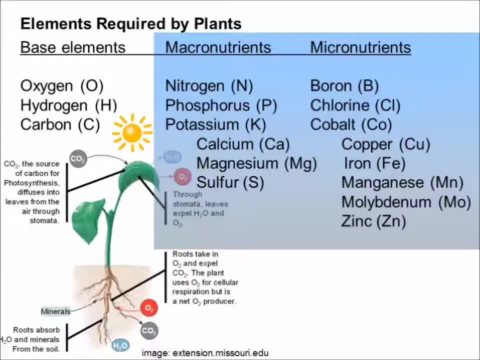 we call macronutrients Nitrogen, phosphorus and potassium Nitrogen, of course, very important in making proteins. And then they need micronutrients that are still important: Boron, chlorine, cobalt, selenium, magnesium, molybdenum and so on. 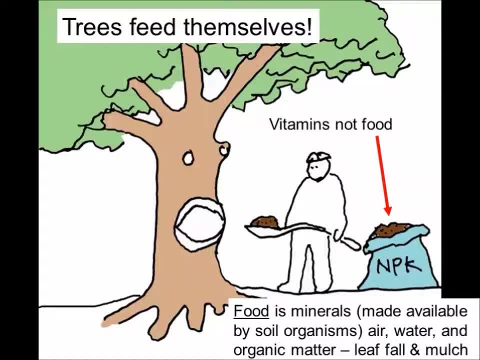 But plants need these nutrients. it doesn't mean that we have to feed them all to them in fertilizers, In fact. obviously, plants have been doing just fine for millions of years, feeding themselves from the soil, And that is the primary way. 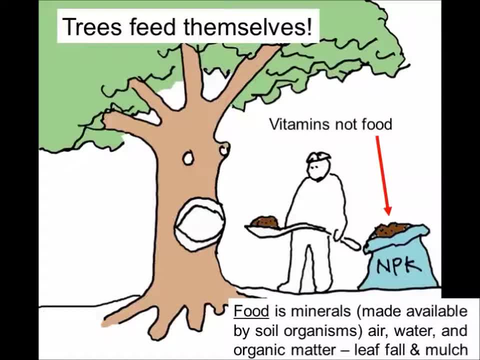 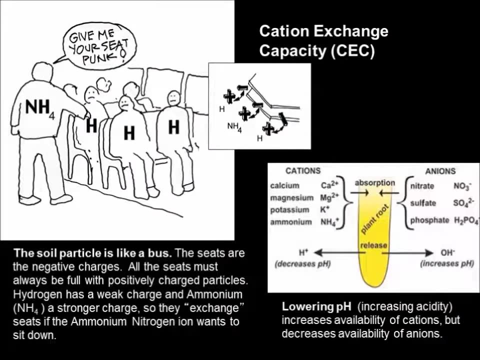 that they get their nutrients. We can supplement those nutrients with certain fertilizers or amendments, but we can never really replace the food from the soil. We can just supplement it- A concept that's oftentimes confusing, but it's important to at least understand. 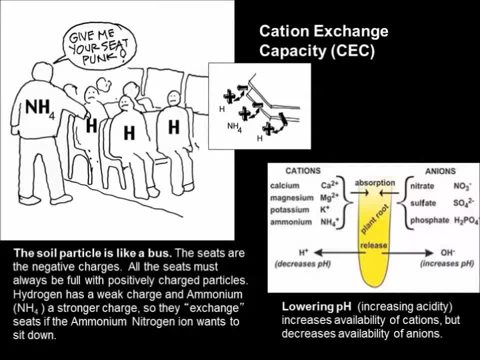 in passing is the idea of cation exchange capacity. Cations are positively charged ions, Anions are negatively charged ions, And a lot of the nutrients that are most important for plant growth are cations: Calcium, magnesium, potassium, ammonium. 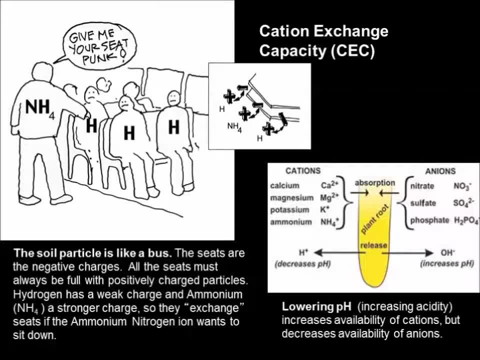 Though obviously some important ones are anions too. But when we talk about important soil characteristics, one of those is cation exchange capacity, And that's basically how many places the soil has to store those positively charged ions so that they're available for plants to grow. 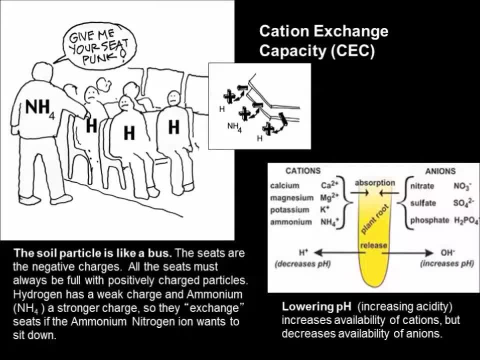 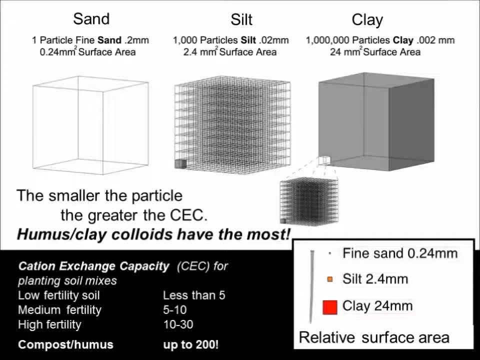 That cation exchange capacity is controlled a lot by how much surface area the soil particles have, what type of particles they are, and also by the pH or acidity or alkalinity in the soil. So different soil textures have different amounts of surface area. 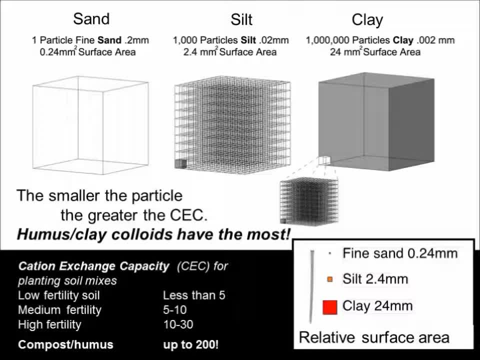 with clay having the most and sand having the least. So clay is inherently has the highest cation exchange capacity. But practically speaking, what makes the most difference in our soils is the amount and quality of the organic matter in the soil, The humus in the soil. 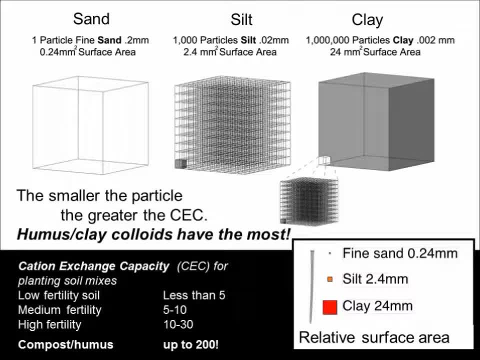 has a huge amount of surface area and a number of chemical bond sites that make it easy to hold nutrients in plant available forms and release them to plants. So it's not just the soil particle size but the amount and quality of organic matter in the soil. 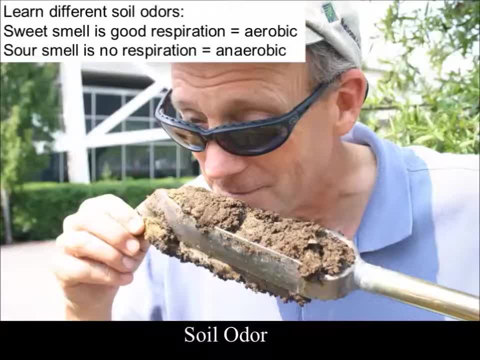 that makes nutrients available to plants And, as we mentioned, we're all familiar with stinky anaerobic soil. My friend and co-presenter, James Urban, here is smelling a soil. You can see that sort of yellow-gray color at the bottom of the soil core sampler. 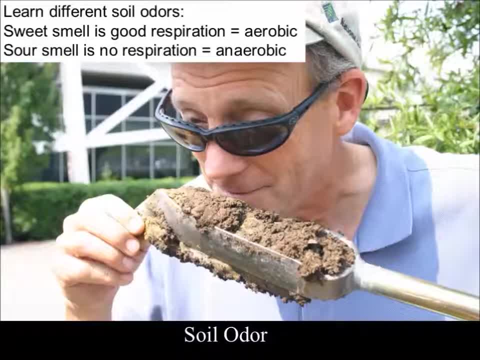 That's typically indicative of an anaerobic soil, in this case, a clay soil that hasn't been allowing a lot of oxygen in And that's going to have that sour smell that indicates an anaerobic soil. Now that can be corrected. 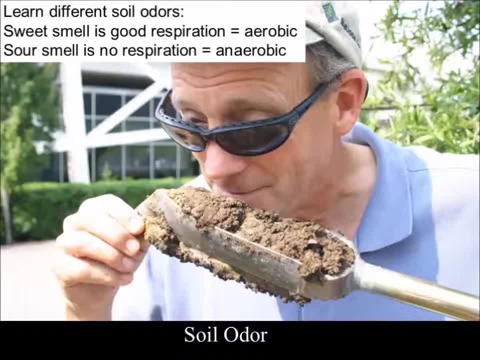 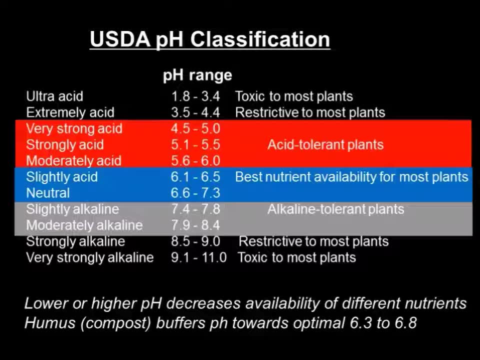 by loosening up the soil and incorporating organic matter. pH is the measure of alkalinity or acidity, with a lower number being more acid and a higher number being more alkaline. And neutral, of course, is exactly pH of seven. It turns out, though. 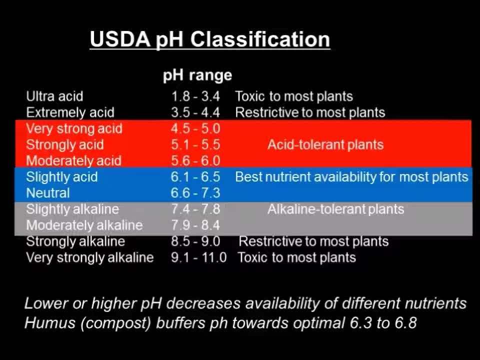 and again. it's because of this cation exchange capacity that the majority of our landscape plants do well in a very slightly acid condition, a range of about 6.3 to 6.8.. So this is close to neutral, just slightly on the acid side. 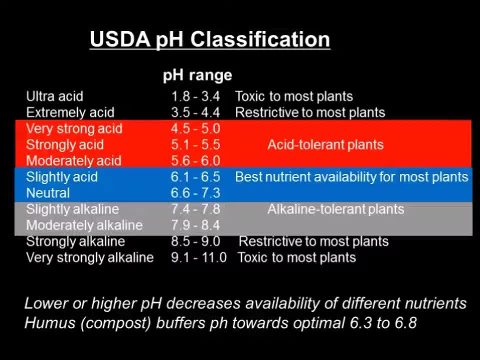 That makes the most nutrients available for most plants Now. native plants in the Puget Sound lowlands that have grown up in more acid conditions may like pHs down in that five to six range. Some alkaline-loving plants may like a higher pH. 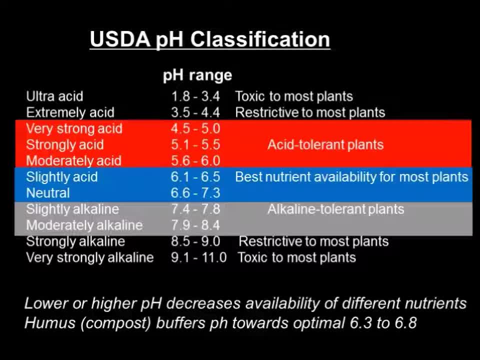 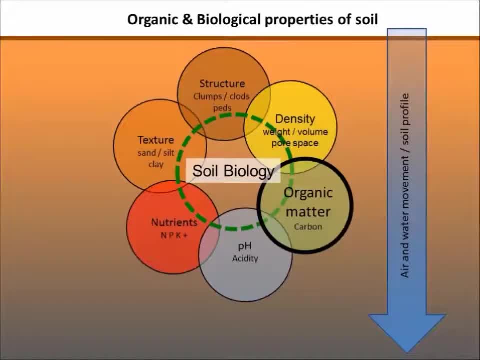 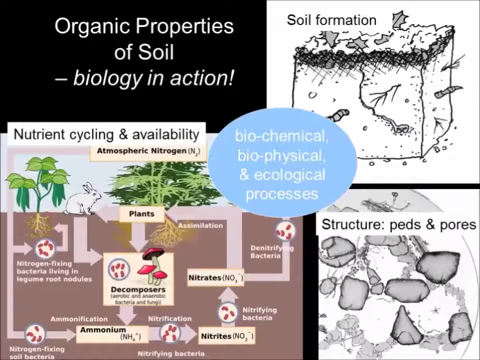 But close to neutral is really what you're shooting for. So that was our discussion of soil chemical properties, And now we'll talk about organic matter and then soil biology. And this is where it really gets quite interesting, because it turns out that the biological properties of soil 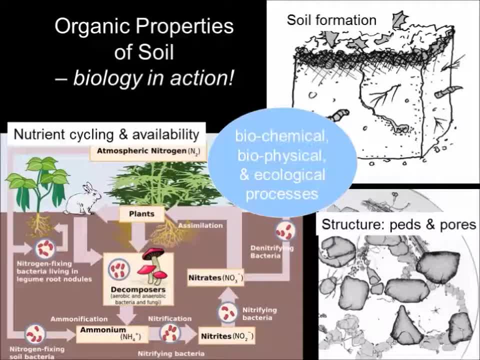 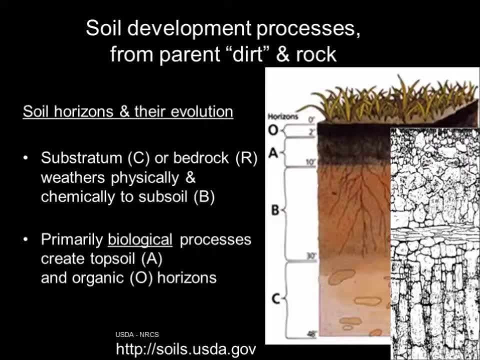 and these biological processes are really what give us the functions that we care about in soil. As we mentioned, native soil has these natural layers, an organic or duff layer on top, a topsoil horizon, a subsoil that's somewhat modified. 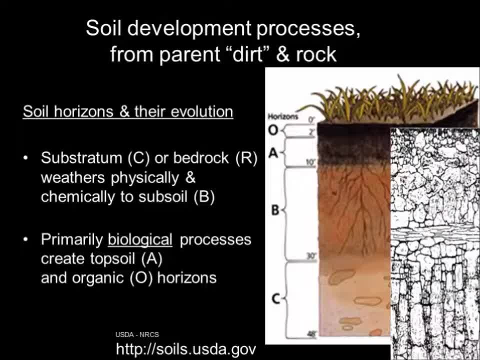 and then the parent material lower down. And the important thing here to understand is that that topsoil is primarily created by biological activities And the processes that create subsoil out of the parent material are a combination of biological and chemical properties, But it's really the biological properties. 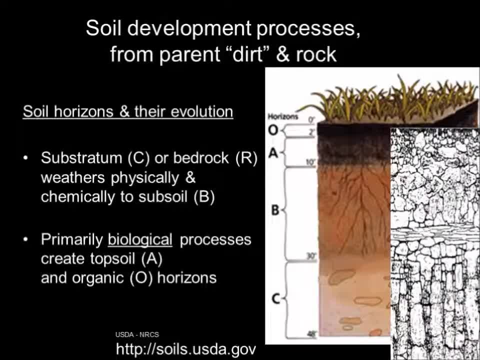 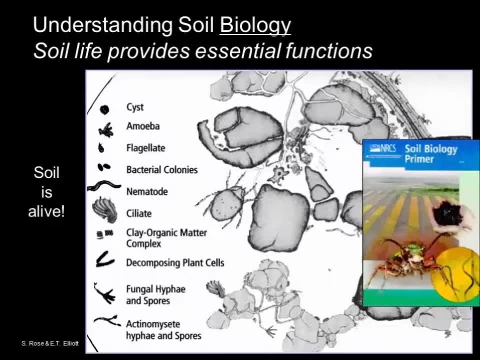 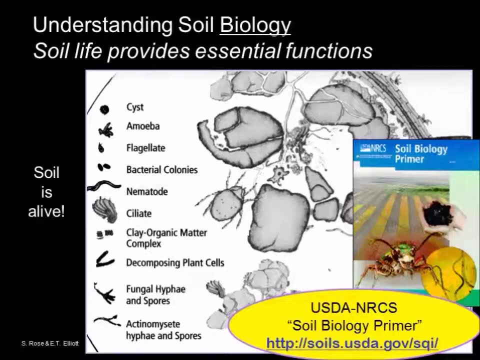 and processes that give us the topsoil that allows for plant growth And, of course, the key thing here is that soil is alive. There's a lot of great resources to learn about soil biology, probably the best being the Soil Biology Primer published by the. 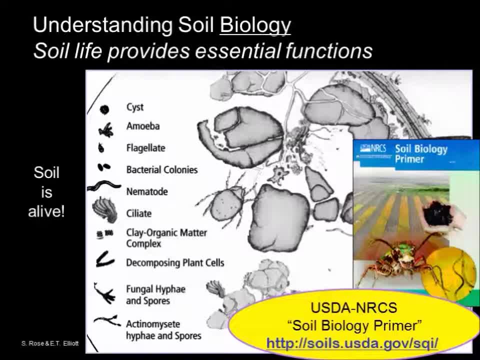 Natural Resources Conservation Service of the US Department of Agriculture. You can find it at this link or just Google soil biology primer, And it's just a great way to learn about some of these organisms and how they provide the function we care about. 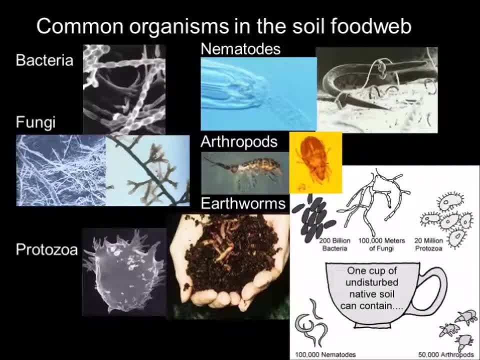 Here's just a few of the organisms in the soil and a representation of how many billions of critters there may be in a very small amount of soil. When all these critters are alive and working in the soil, we end up with healthy soil. 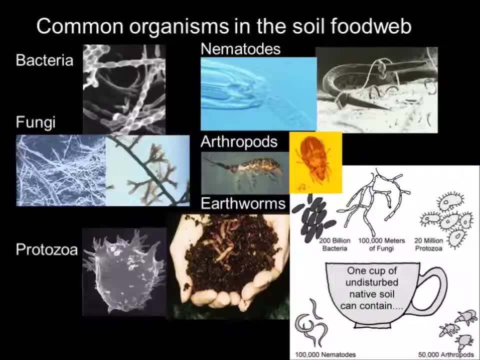 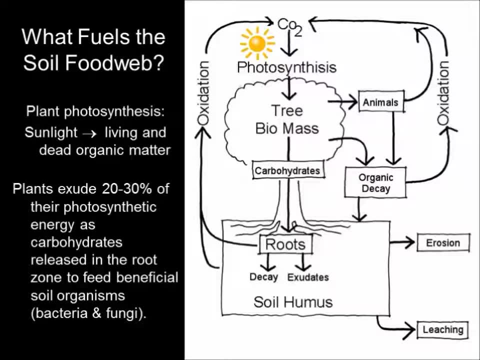 which leads to healthy plants that are easy to care for, have few pest problems, need less irrigation, need less chemicals and so on. And this soil food web, of course, is fueled by the sun and by plants photosynthesizing and then those organic materials. 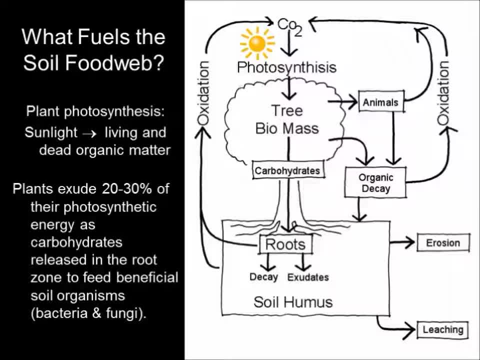 being released into the soil, either when the plant dies and decays, or leaves fall and decay, or all plants- terrestrial plants anyway- exude a lot of the carbohydrates that they create through photosynthesis into the soil around their roots, And they do that in order to attract. 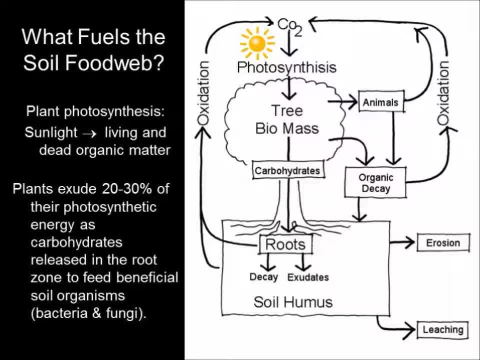 and support the beneficial organisms, both bacteria and fungi, that they depend on for disease protection, for processing nutrients and bringing them to them in plant-available forms, and so on. So just like we depend on the bacteria in our intestines to help us digest food, 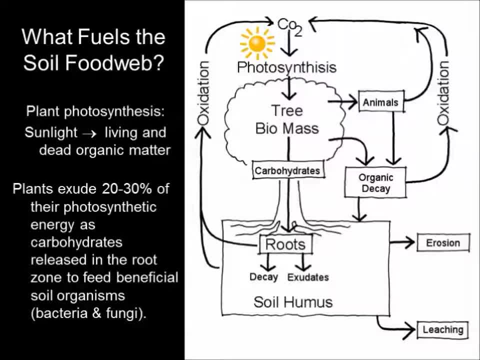 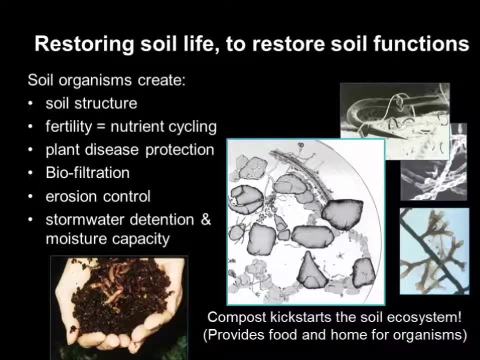 plants depend on bacteria and fungi to help them grow and they actively release carbohydrates into the soil to feed those beneficial organisms. So, as I mentioned, these soil organisms create the functions that we care about in the soil, the things that us humans really want to see. 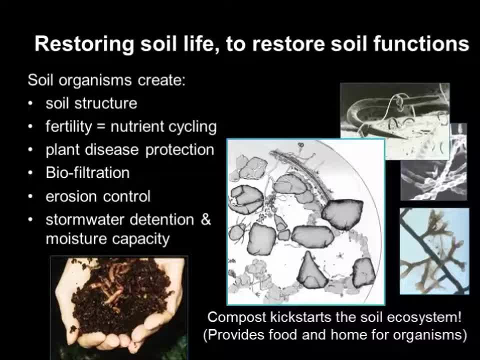 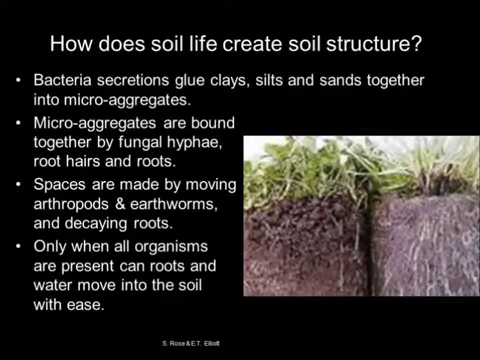 in a good, healthy soil and also the same functions that are provided in a native or natural soil condition. Soil structure is created by bacterial secretions gluing the tiniest particles together into microaggregates. Those microaggregates are bound together then. 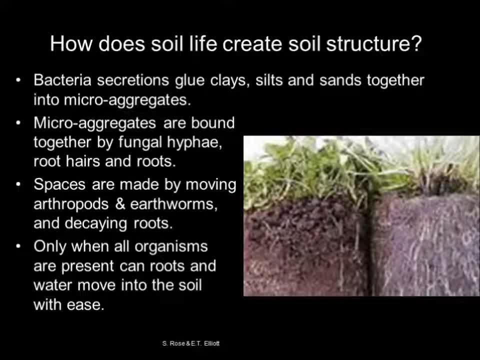 by fungal hyphae or little hairs and root hairs and roots. the spaces are made by moving arthropods or joint-legged critters and earthworms and by roots decaying and leaving spaces, And when all those organisms are there together. 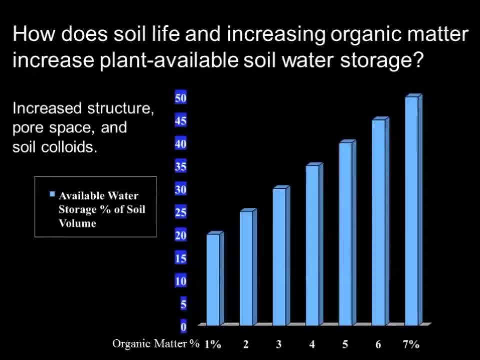 they create soil structure. Soil life also increases the organic matter in the soil and that increases the plant-available water storage in the soil. So you can see how going from the soil. you can see how going from 1% organic matter in the soil up to 7% in this particular example. 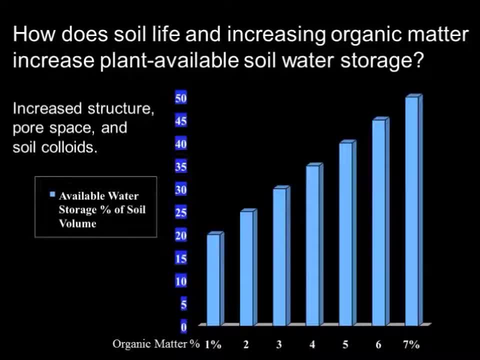 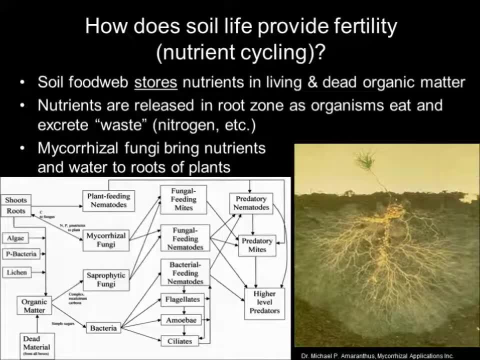 just about doubles, or more than doubles, the plant-available water storage. This is an important reason to incorporate organic matter into soil. Soil organic matter and soil biology also contribute to nutrient cycling in the soil, As we mentioned, the organic matter can hold a lot of nutrients. 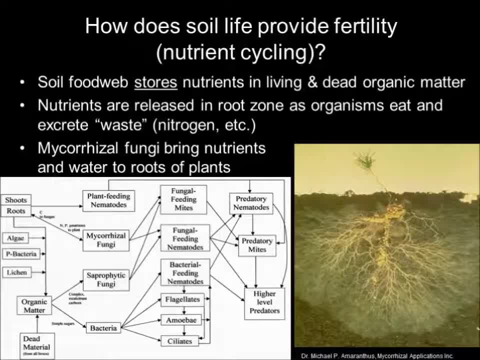 And all these organisms in the soil as they feed on each other. they take in what they need to grow and they excrete what they don't need, And the things they excrete are things like nitrogen, potassium, phosphorus. Sound familiar. 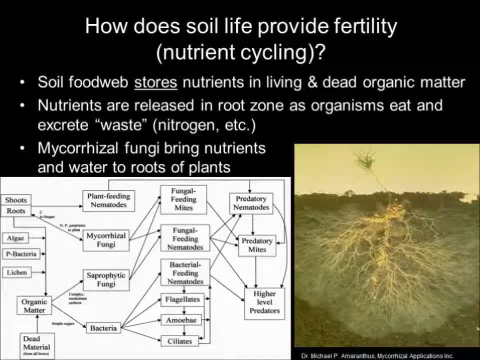 The plant nutrients that we need And they excrete them in forms that plants can use. And also plants develop these webs of mycorrhizal fungi. Mycorrhizal just means root fungus that grow from the plant roots out into the soil. 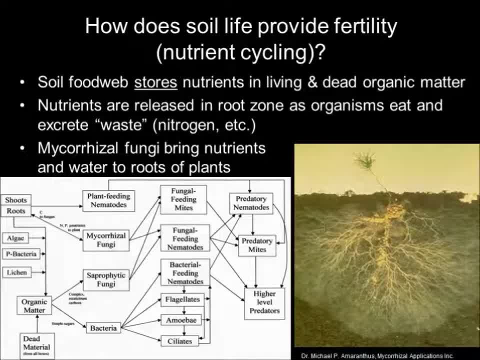 You can see a few-week-old pine seedling on the right here with its mycorrhizal webs starting to grow out into the soil. In Oregon we've measured these mycorrhizal webs going for miles between trees. They bring nutrients to plants. 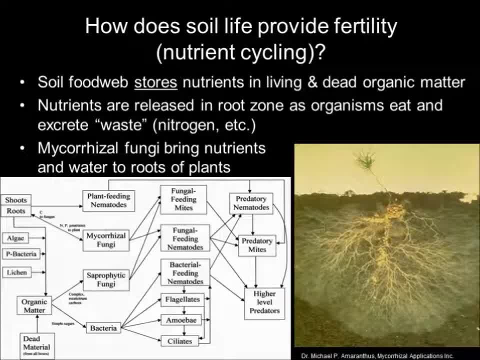 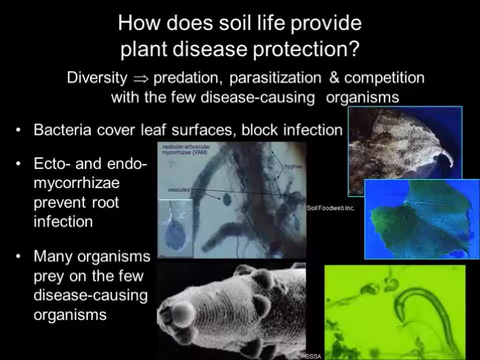 they bring water to plants and they protect plants from the few disease-causing organisms. These organisms, by coating the roots and the leaves, prevent them from being invaded by disease-causing organisms. And these beneficial nutrients are the ones that actually make the natural soil organisms. 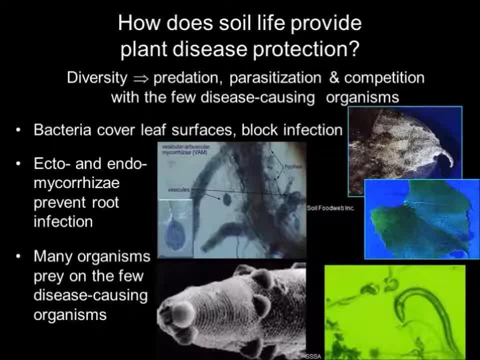 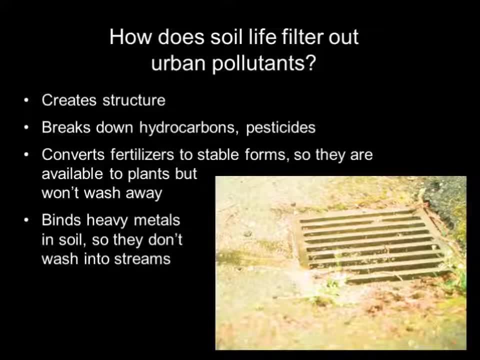 actually prey on those few parasitic or disease-causing organisms so that it's difficult for the parasites to get going in a healthy soil. Soil organisms also have many different biological biochemical pathways that they can use to break down and actually use as food many of our common urban pollutants. 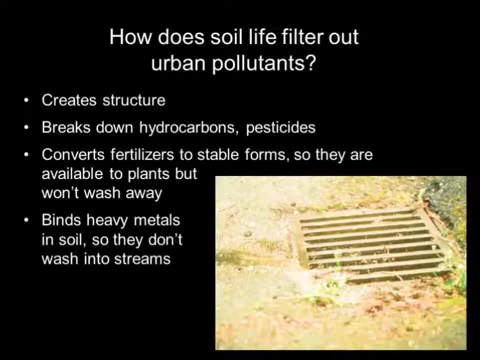 Things like oils and greases and pesticides. they break them down and eat them. They convert fertilizers to more stable forms so they stay available to plants longer and aren't washed off into our waterways, And they bind heavy metals in the soil. 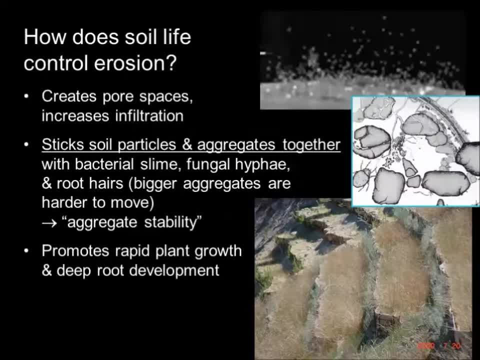 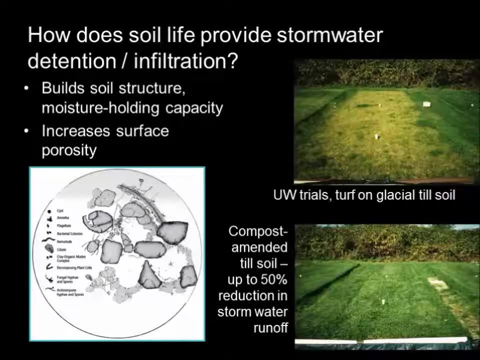 so they won't wash off into the streams. By creating soil structure, these organisms also stick the soil together and, of course, help grow plants that prevent erosion. So the soil biology is very important in preventing soil erosion And by creating structure in the soil. 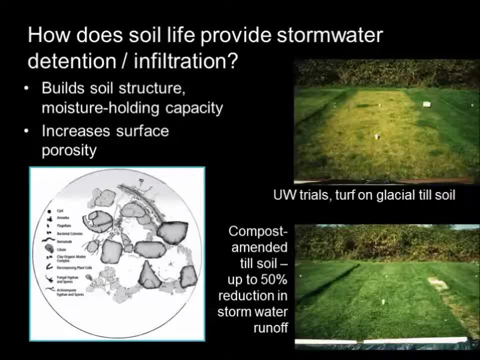 and pore space. the soil organisms allow for water to flow into the soil during heavy rainstorms and reduce stormwater runoff, and also to hold moisture in the summertime, so it's available for plants. Fortunately, you don't have to be a soil scientist. 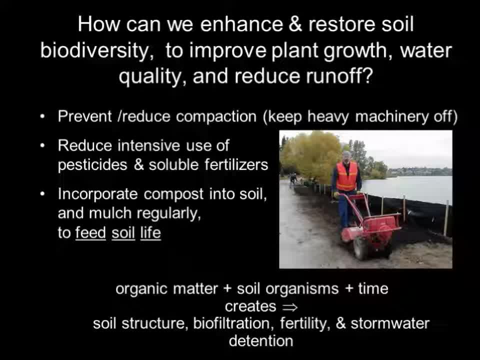 to understand how to improve the soil. All you need to do is break up compacted soil and incorporate some good quality organic matter, as my friend Lonnie is doing here by Green Lake, tilling some compost into a highly compacted soil. former running path. 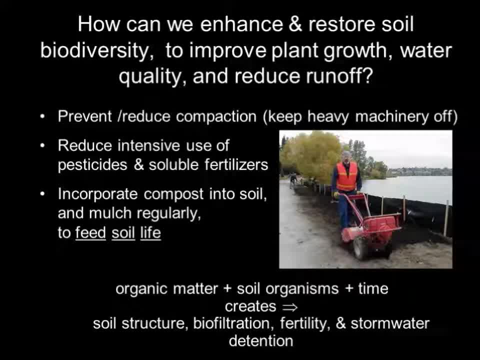 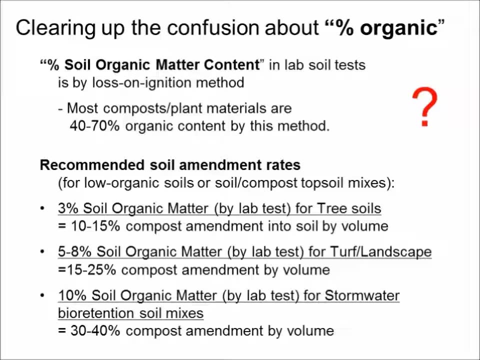 and successfully growing plants in that soil. So it's not rocket science: Break up compacted soil, get good quality organic matter in it, and the soil organisms will move back in. When we see soil tests, we can oftentimes be confused by 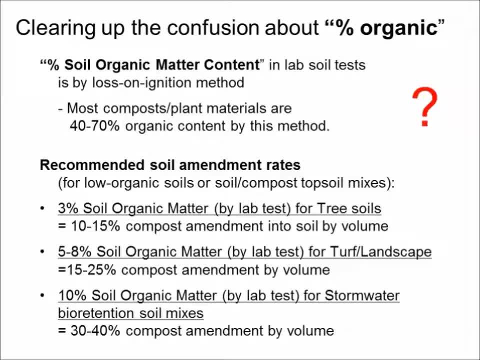 the use of the term soil organic matter in those soil lab tests. So this slide is attempting to explain that Obviously, organic matter is just stuff that was formerly living or alive. So organic matter in the soil is all the growing critters and all the other brown decomposing stuff in the soil. 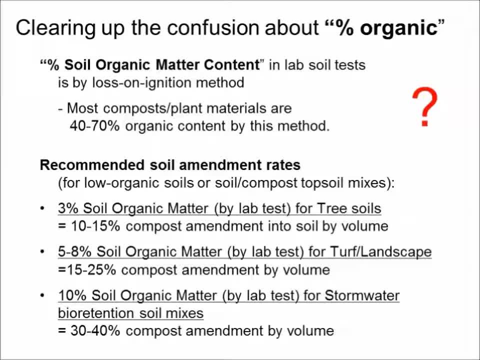 So, for instance, a compost would be 100% organic matter by that common sense use of the term. However, in a lab test for organic matter, most composts would be 40% to 60% organic matter, And that's because what the lab does is. 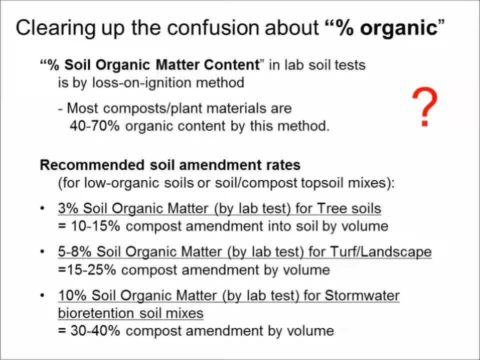 it dries the sample out, it weighs it and then it heats it up until it burns off most of the carbon, its carbon dioxide, and weighs the remaining ash and the carbon that didn't burn off And the difference it calls percent soil organic matter. 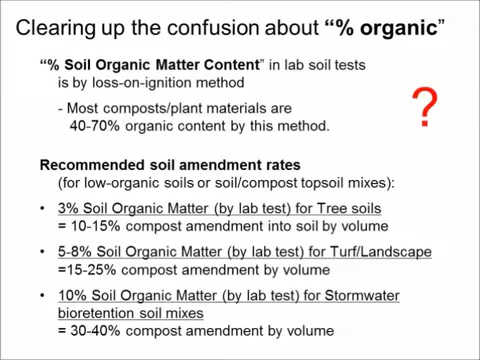 So by that test we mentioned, most composts are 40% to 70% organic matter And most soils may be just a few percent organic matter. And when we amend soils to improve or restore organic matter it takes quite a bit more compost. 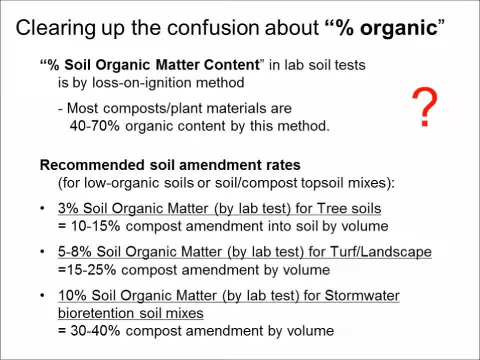 to increase the soil organic matter by a percent. So for instance, for, say, a sandy soil with no organic matter, to get that up to about 3% organic matter by the lab loss on combustion test, we'd have to add about 15% compost by volume to that soil. 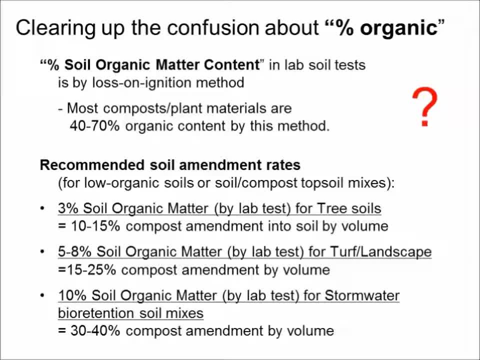 To get 5% to 8%, which we'd prefer for most turf and landscape installations. we'd want to add about 25% compost by volume And to get 10% organic matter by the lab test which we like for stormwater bioretention swale mixes. 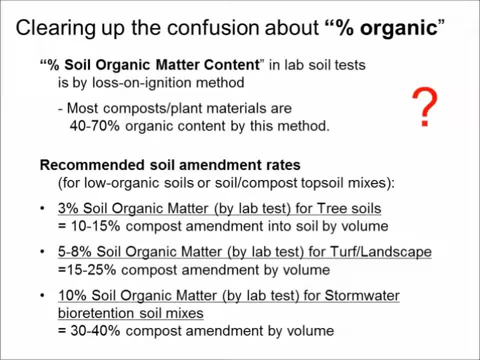 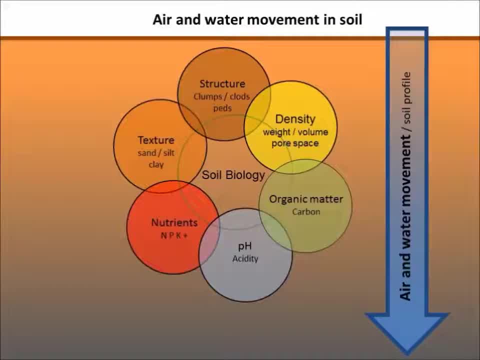 you would need 30% or more compost, 30% or more compost by volume in that soil. So that's our discussion of soil biology. Now we're going to talk a moment about how air and water move through soils, And then we'll kind of put this all together. 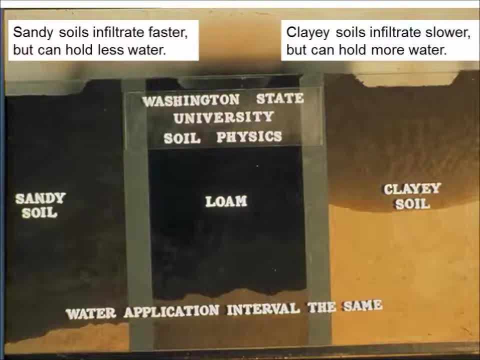 Obviously, sandy soils can soak up water more quickly, And anybody who's been around beach sand, as compared to heavy clay, has seen rainfall on it. The rain is absorbed quickly on the sandy soil, whereas it may sit on the surface on a silty. 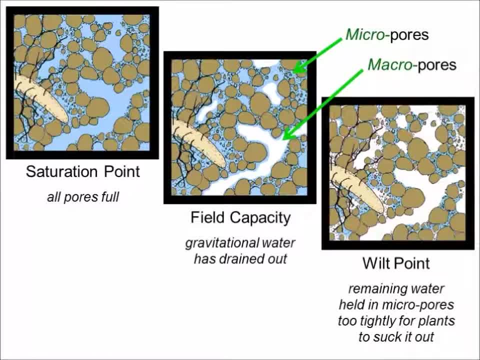 or certainly on a clay soil. Scientists talk about three different levels of water in soil, And it's good to know about these terms and to understand what they mean, because they can help you understand how you can soak up and store water usefully in the soil for it to be available for plants. 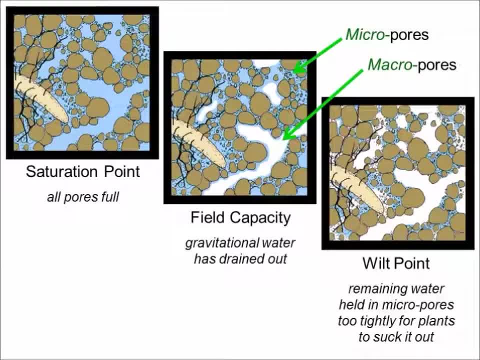 The saturation point is when all the pores, both the tiny microscopic pores and the macropores pores you can see, are full of water. So saturation point is just completely full of water. Field capacity is when the water has drained out of those macropores. 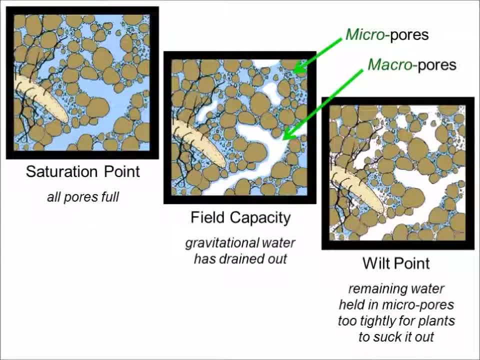 but it is still adhered by surface tension in the micropores and the surface, So there's actually still a majority of water is still held in those micropores. The wilt point refers to plant growth And the wilt point is where the remaining water. 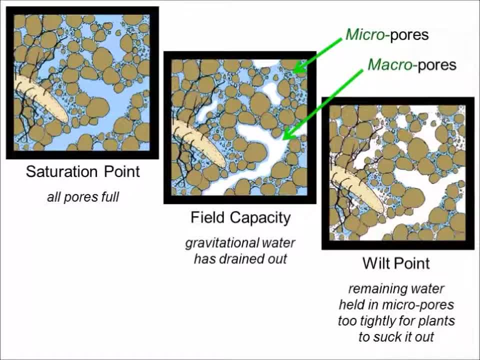 is so tightly held by surface tension in the smallest pores and surfaces of the soil that the plant just can't suck any more water out of it. And that's where that mycorrhizal web can often help, because the fungi in the mycorrhizal web 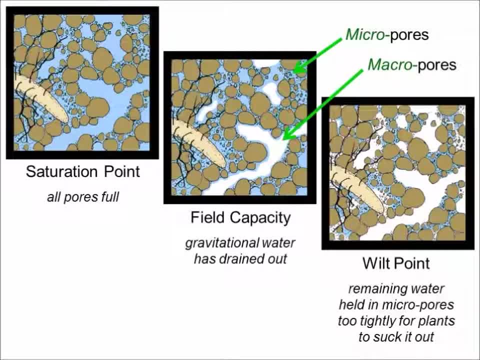 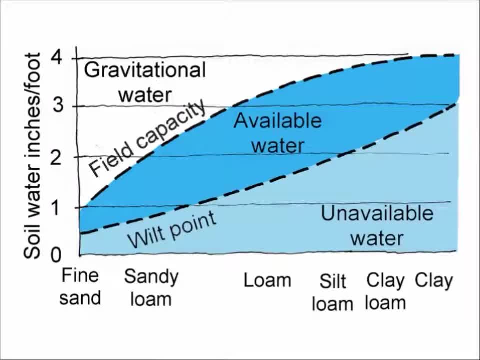 can actually access water down to a lower wilt point, oftentimes than the root hairs of plants. The plant available water is the difference between the field capacity and the wilt point of the soil. So at the top you see gravitational water and that's what just drains out after a rain. 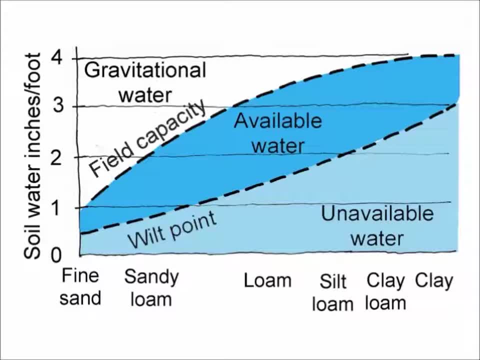 And then. so that would be like in the summertime: we had a rain and then a field. A few days later, most of the gravitational water would have flowed down into lower levels and we would be at field capacity, and then the plants would gradually use that water. 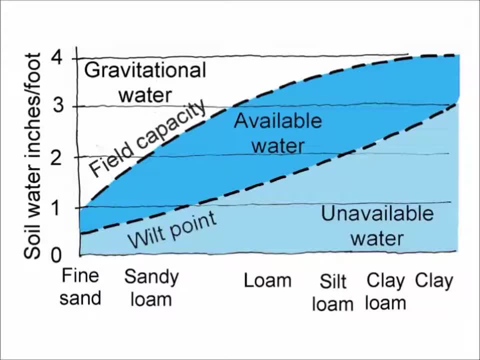 down to the wilt point, the point at which they can't suck any more out. And, as you can see, typically in soils we have more plant available, water in the soil, that has more silt or clay in the soil as compared to sand. 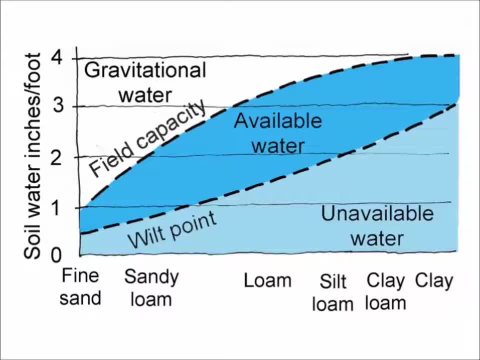 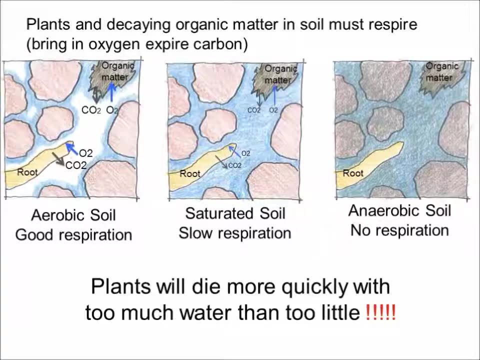 However, the important thing is that we can greatly increase this plant available water by incorporating organic matter into any of these soil types and building soil structure. Plants also need to breathe in the soil, so they need those pore spaces and that's also why we want our soils. 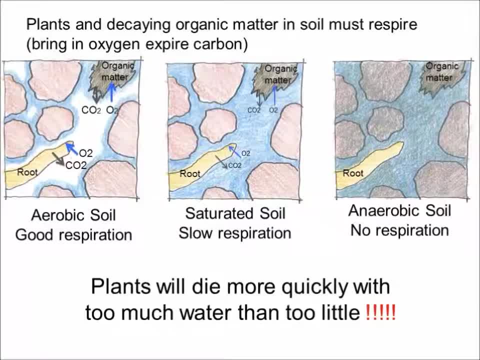 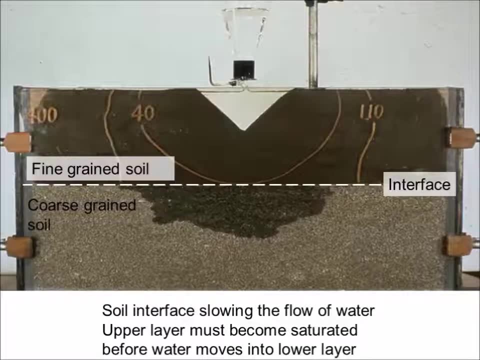 not to stay saturated all the time. We want to have good drainage in the soil because that reduces when the soil is saturated. that reduces the gas exchange. The other thing we want to avoid in our soil is what soil scientists call interfaces, and that is just a sharp horizon. 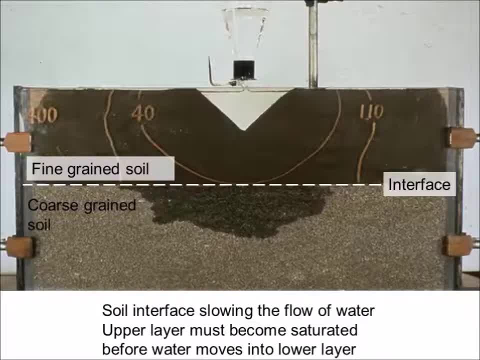 between soils of different particle sizes, different textures. So in this case, we've layered a fine-grained silt soil on top of a coarsely grained sand soil. and it's an odd thing, but it's true that when we soak water in from the surface, 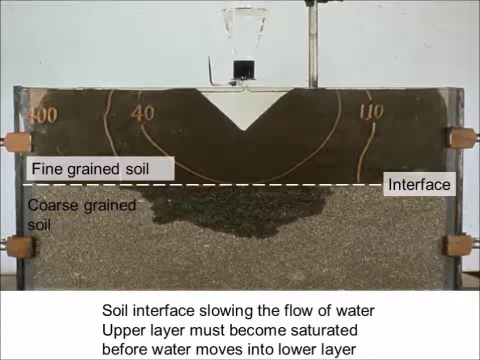 into that fine-grained soil. you would think once it hits that sand, the soil boy, it's just going to soak through really quickly. In fact, because of that interface, that sharp borderline between the two, it's difficult for water to penetrate. 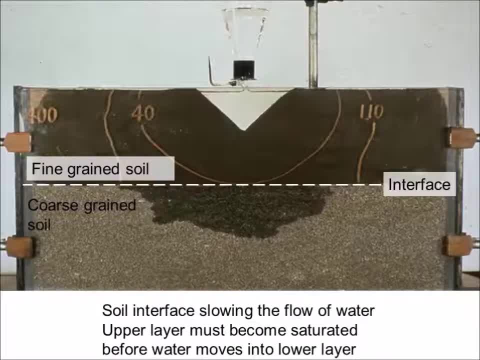 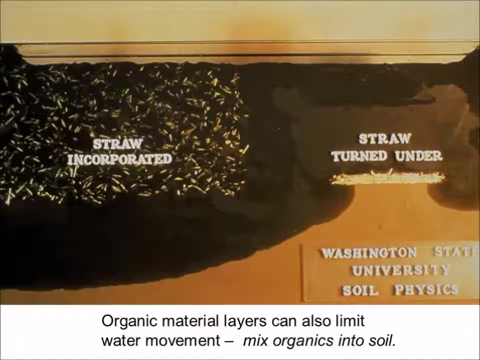 even into that sandy soil. So we want to avoid interfaces. We want to mix up the soil when we're placing layers of soil, rip it or otherwise mix it up so we don't have those sharp interfaces. Here's just an example where we had straws. 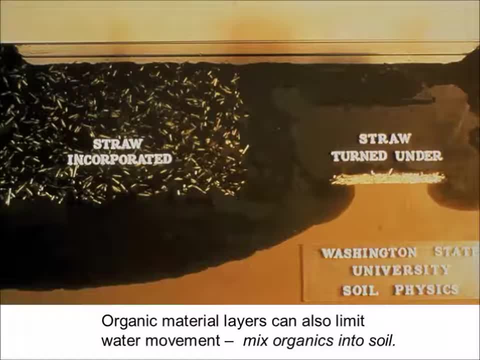 or organic matter just kind of left near the surface, as opposed to the same straw that was tilled into the soil. On the right you can see that sharp interface layer of straw and water really isn't penetrating through it, whereas when it was incorporated into the soil 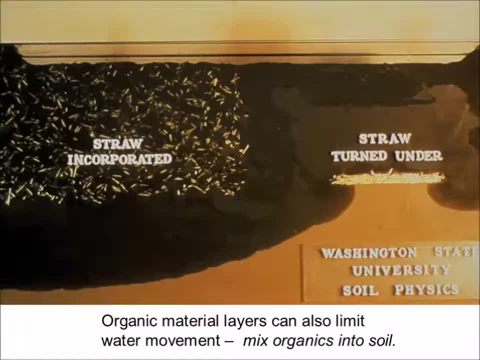 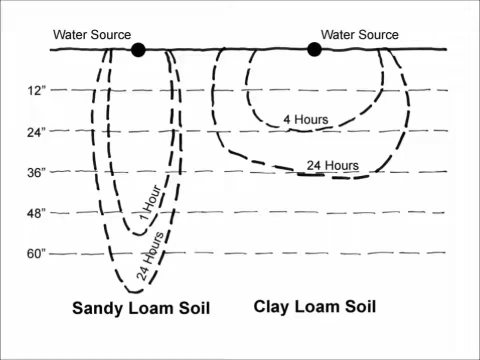 water penetrates much better, And we do this by tilling organic matter into the soil or, in a turf system, by aerating and again mixing the organic layer somewhat into the soil. Here's just an example of penetration rates, again that we talked about, in a sandy loam soil. 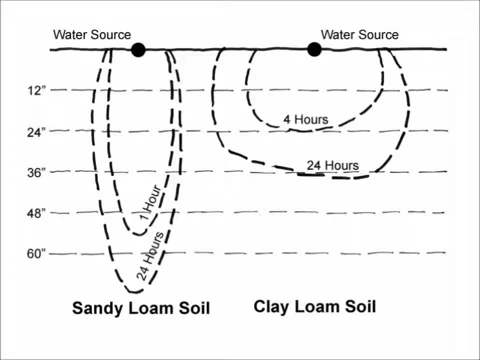 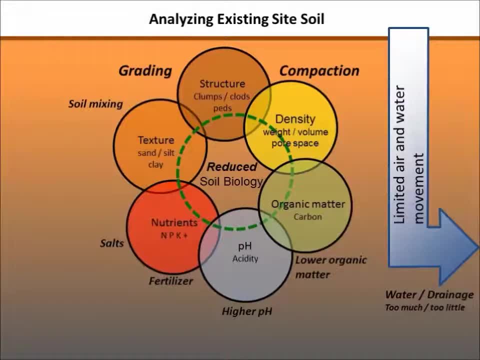 how quickly and how deeply it penetrates as compared to a clay soil. The clay soil will hold more water, but it penetrates more slowly. So now we've talked about soil physical characteristics, chemical characteristics, biological characteristics and organic matter and air and water movement. 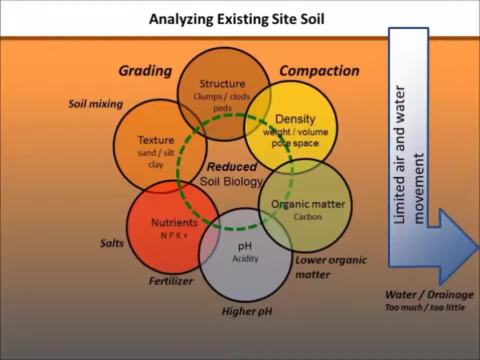 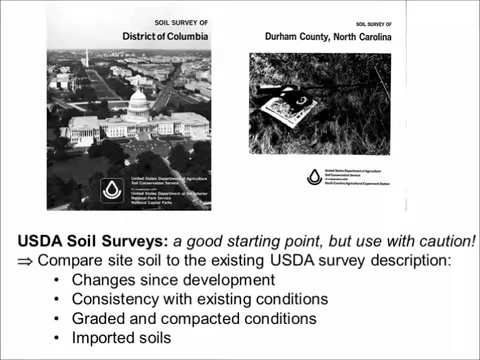 And now we're going to talk a little bit about how we analyze or look at our site soils. to put this together and put it into useful terms, First of all, you can look at your agricultural soil surveys, and particularly if you're working in an undisturbed soil condition. 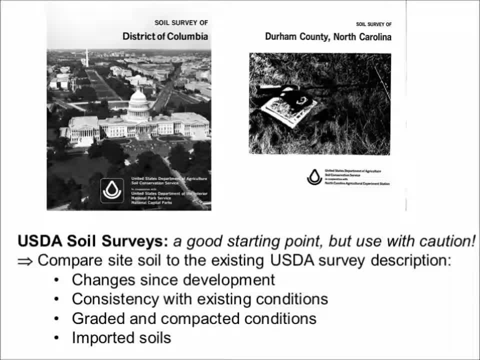 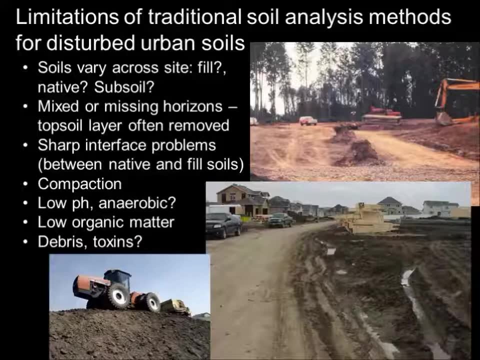 those can be very useful, but they're kind of a gross level and if your site has been disturbed they may not be that much use to you Really. what may be more use is to actually dig in and look at the soil, see how it has been disturbed. 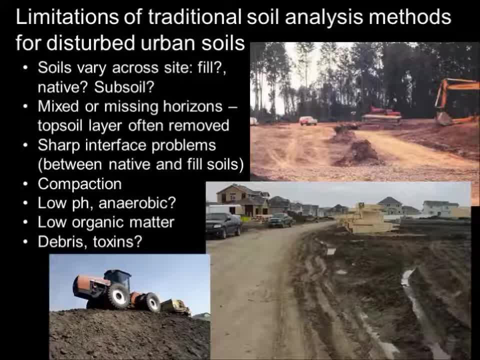 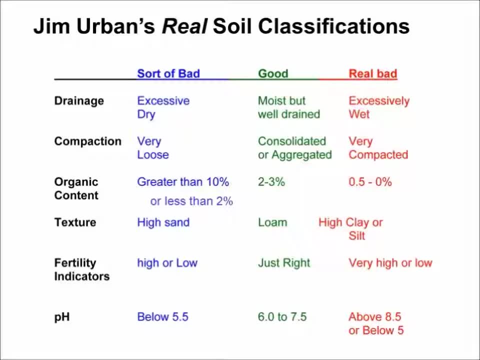 look at the history of the site and see whether some of these various characteristics we've been talking about have been changed over time. So here again, my co-presenter, when this was originally presented to the ASLA, Jim Urban put together this chart of some of the conditions. 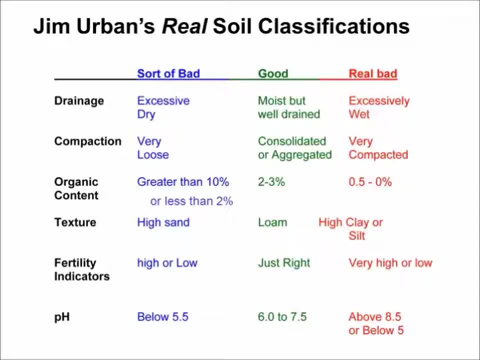 we actually tend to run into in landscapes and what we can live with and what we can't. So the sort of bad- the good is what we'd like, the sort of bad is what we usually run into and the real bad is it may be time to do some serious modification. 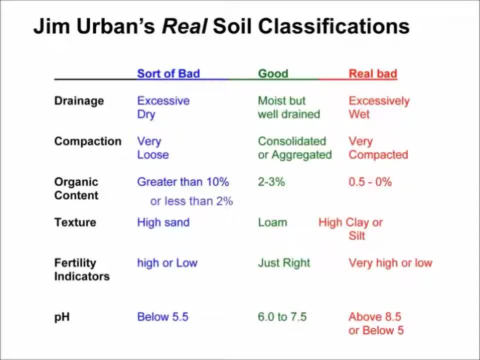 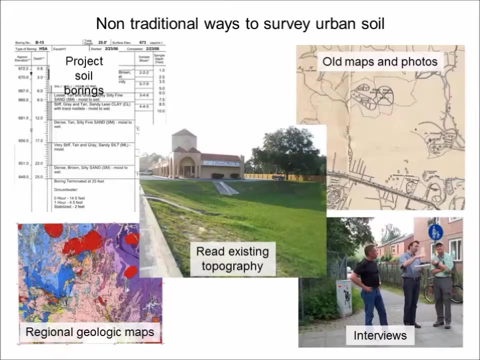 of that soil. So this table is just an example from the standpoint of drainage, compaction, organic content, soil texture, fertility and pH, things that we can live with and things that may be very hard to grow plants in. So some of the other ways. 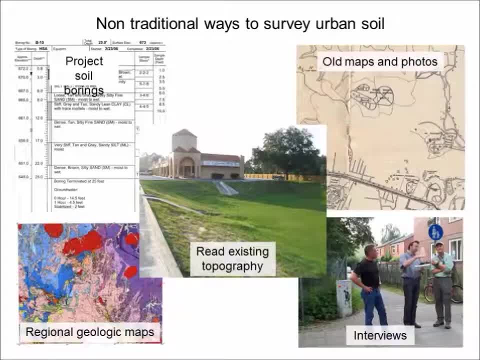 to look at this soil are to look at soil borings- and there may be, those may exist- whether they've been done for hydrologic regions. You can look at the existing topography to see what may have been modified- old maps and photos- and then, particularly talking with people, 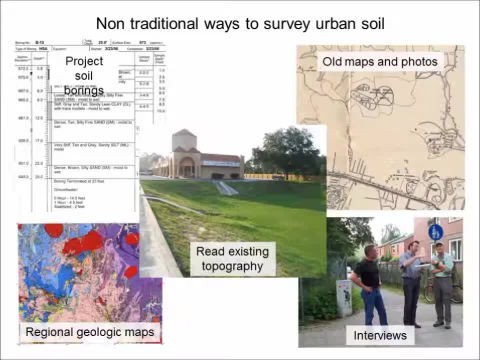 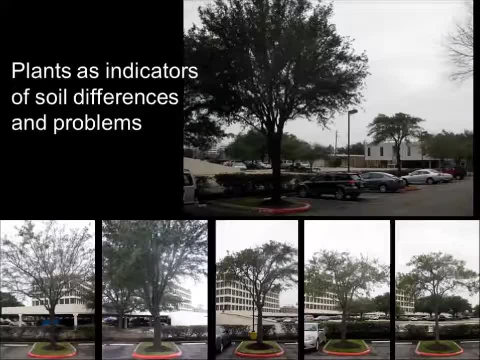 who've been around on a site for a while to know how the site may have been modified over time. You can also use plants on this site as indicators, For instance, the trees in this site in the different plots between the parking lot areas. 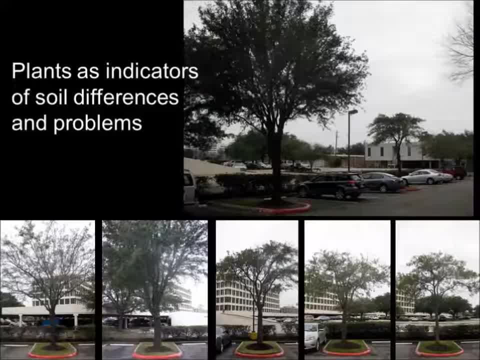 some are growing well and some aren't growing well and that is going to tell you a lot about the soil conditions under that site. Then you could move in with your soil core probe or that soil dutch auger and make some core holes and see really what's going on. 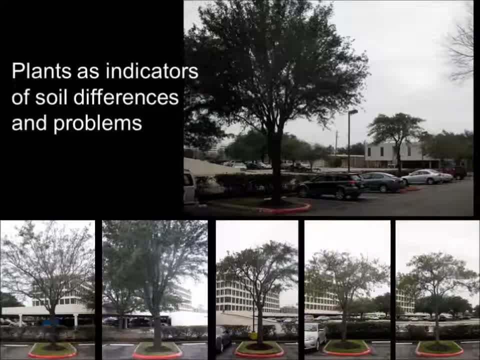 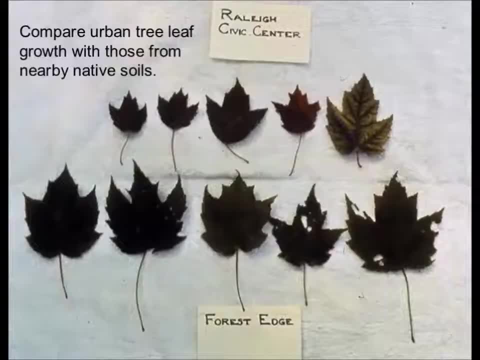 underneath there. Typically it's going to be compaction, loss of organic matter or lack of access for the tree roots out to the surrounding soils. You can also look at similar species in adjacent soils and compare the leaf growth, For instance our leaf at top right here. 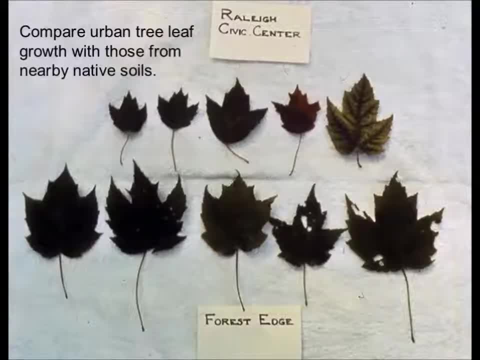 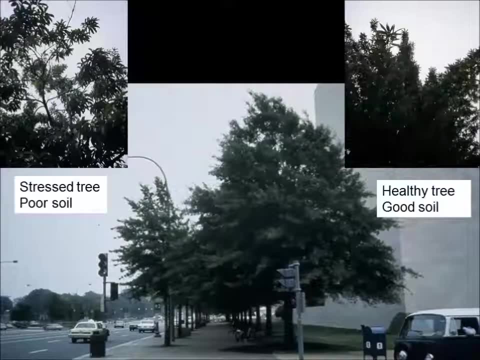 may indicate some nutrient deficiencies in that soil. Here again, same species of trees. The row on the right has access to a much larger soil area than the row on the left, and they are growing much better. The row on the left will probably eventually die. 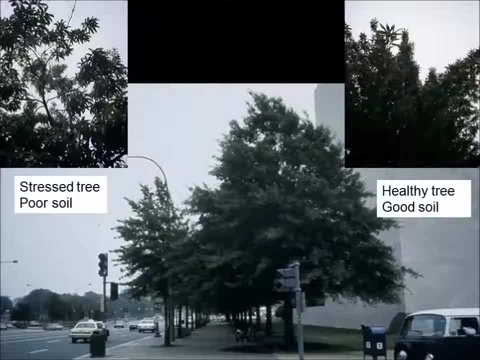 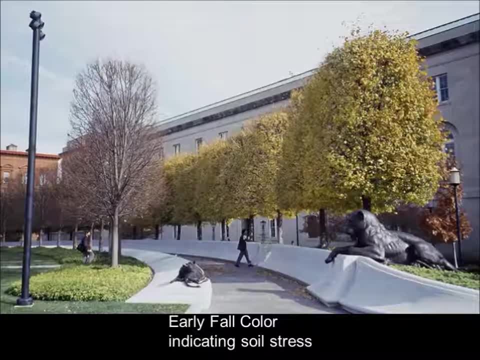 The row on the right will be able to grow to mature size and stay healthy for many years. Early fall color is also an indicator of soil stressors and again, you can use the leaf color things that are happening in the leaf veins to get an idea. 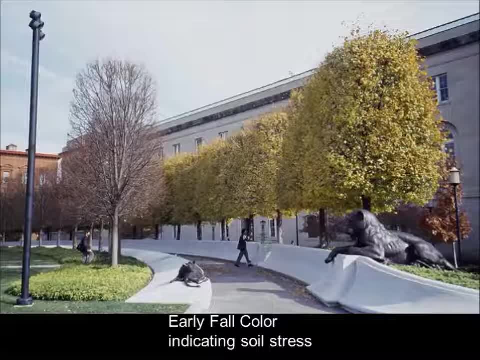 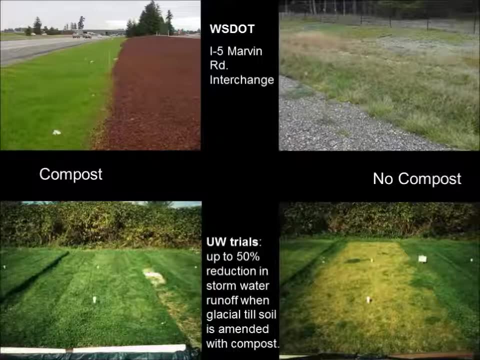 of specific nutrient deficiencies too. Here again with turf. on the left you can see examples in a highway interchange, in one of our soil plots at the University of Washington with soil that's growing in a compost amended soil and doing very well, Whereas on the right you have turf. 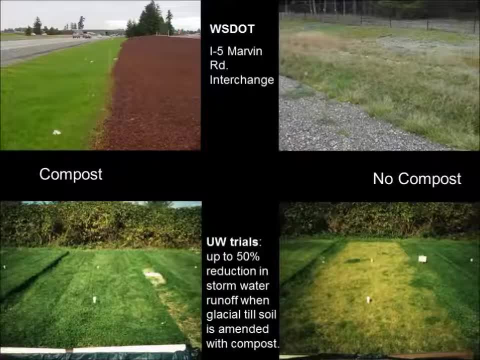 same kind of grass planted in the highway interchange and down in the test plot bottom right, and several years later in both cases you can see very poor turf development, a lot of weed, invasion, sparse, very drought damaged those soil biological properties, structure, nutrient exchange etc. 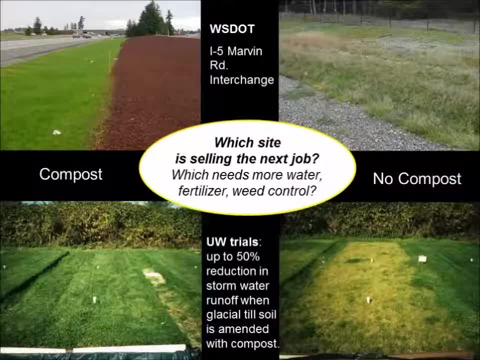 While we talk about soil health for a variety of reasons, it's important to just think about which site is selling the next job. It turns out that treating soil right is really cost effective because it helps you be successful, have successful plant growth. Here we are again using that. 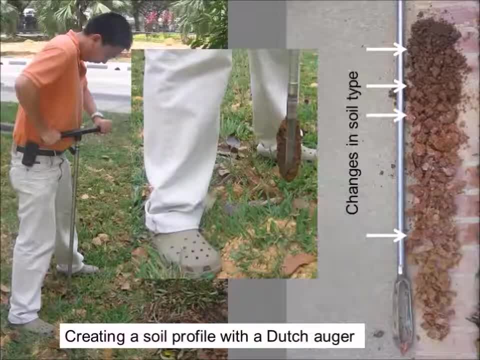 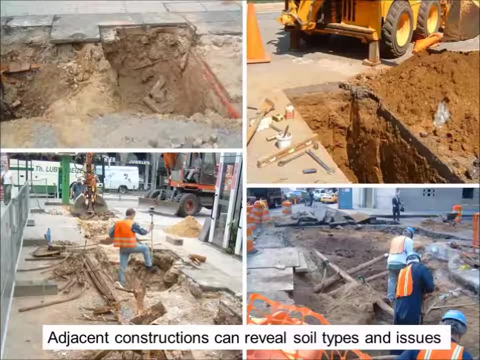 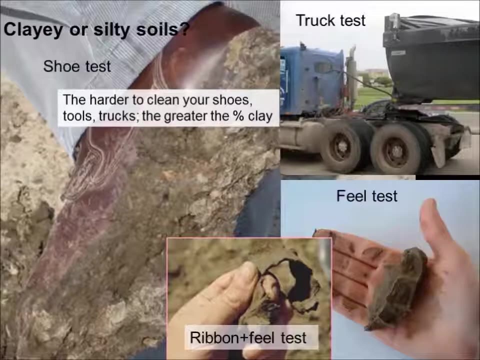 Dutch Auger, to create a deep soil profile and look at a site. You can also often times look at soil excavation holes to be able to see some of these soil horizons and what's going on. And just again, the shoe test, you know. 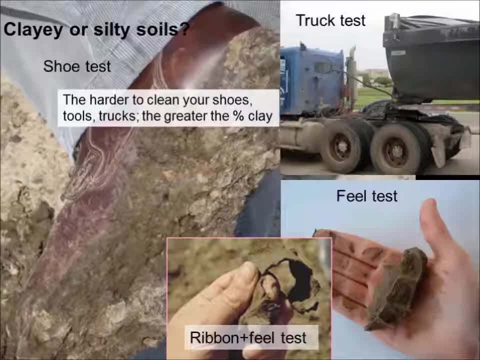 you walk across the site and if it really sticks to your shoes, it's got a lot of silt and clay. and if it really sticks to your shoes it's probably got a lot of clay and then you can do that soil ribbon test and bottom center here. 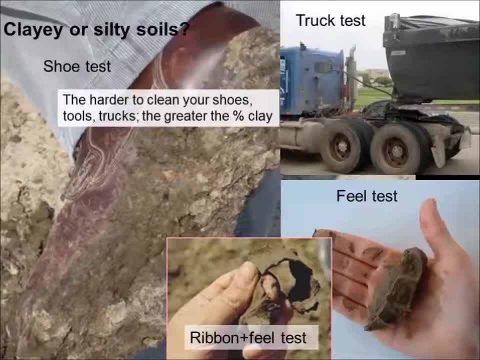 you can see an example of a very clay soil where we get a long ribbon out of that ribbon test. This can be a heavy soil and difficult to work with, but it can be improved, as we'll talk about in the next section The concept of getting a reference soil. 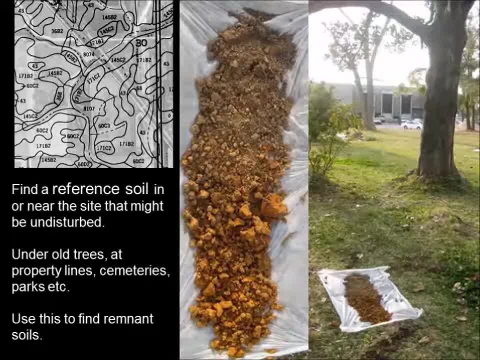 a good quality soil that you can compare to is important. Looking for a place- perhaps a native soil where trees have been growing for a while, where you can take a soil that you're shooting for and compare that to your site soil conditions and give you an idea of 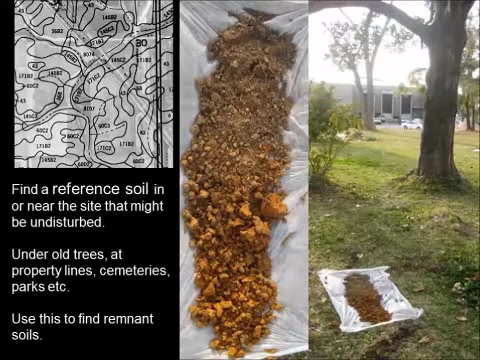 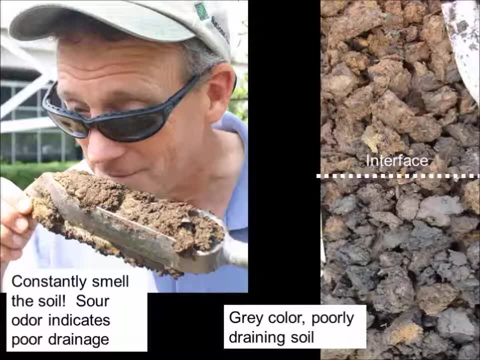 what you're shooting for and restoring that soil is important. So reference soil is an important concept. And again, smelling the soil, looking for interfaces, look for differences in soil color that indicate an anaerobic or poorly drained soil, and then start to make your own soil search. 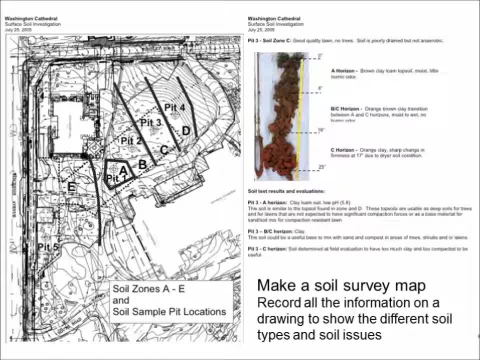 or survey map, combining all this information into your map of the site, your soil core, probes, maybe some historic information you gathered, maybe some soil tests you talk about in the next section, so sending it off to a soil lab and getting soil test results, all these things, combining these on your 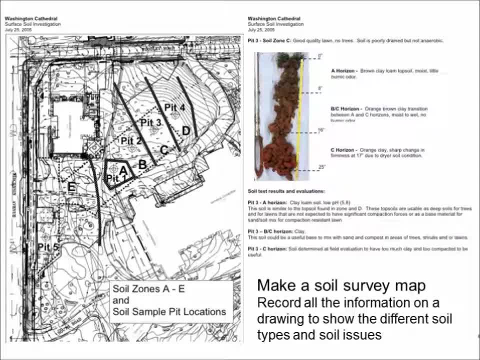 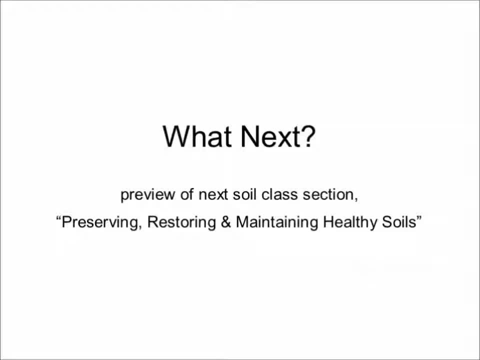 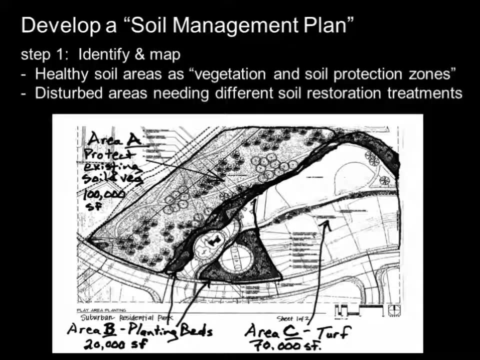 soil sample map to describe the site more completely. So that's our soil science class. in the next part 2 of this soil class- preserving, restoring and maintaining healthy soils- we're going to focus on strategies that you can use for protecting and restoring soils. 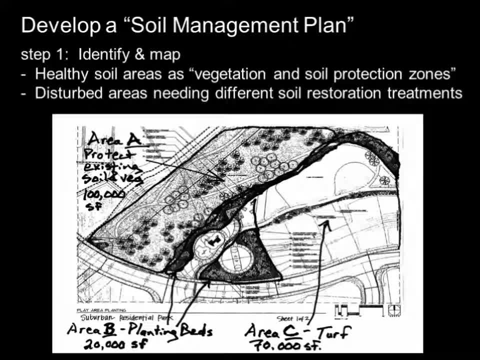 on sites, and a key strategy is going to be taking our soil survey information and then creating a soil management plan that indicates areas that we're going to protect from development, from tree and vegetation removal, compaction, scraping the soil off, and then areas that we are going to disturb. 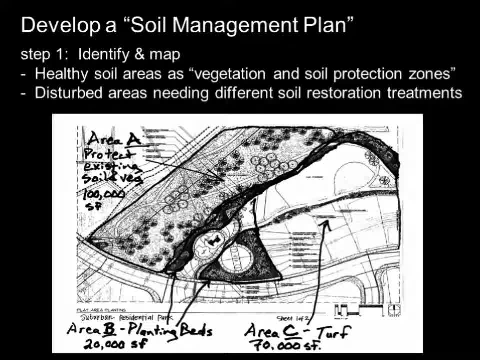 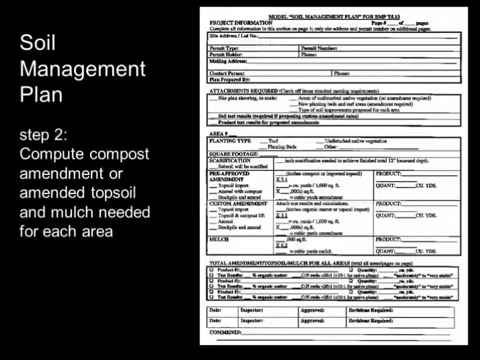 scrape off, compact, whatever how we're going to restore, decompact, incorporate organic matter and so on, in order to end up with an appropriate soil condition for whatever we're growing: turf, planting beds, restoration projects, etc. and, together with that, soil management plan. 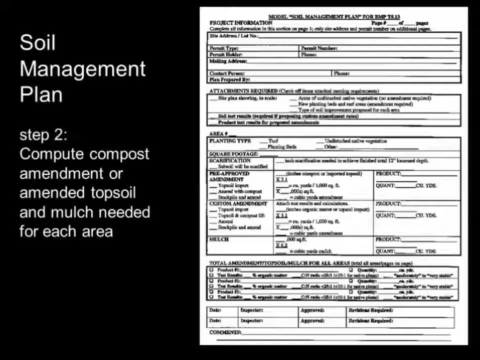 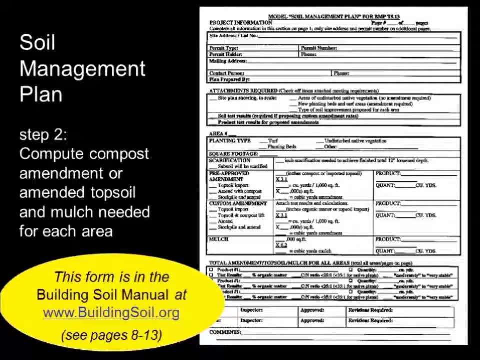 or drawing. we're going to develop a simple narrative plan that says, for these different areas, we're going to protect this area in this way, we're going to restore this area in this way, with this much amendment, or amended soil, etc. This information is all available, as you'll see.